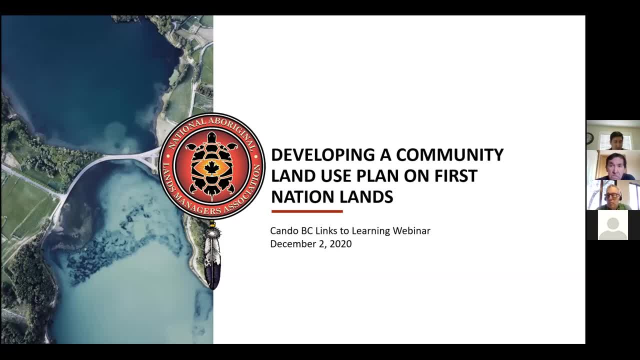 and doing land management activity there And, prior to that, working with other industry planning related fields. This webinar is a bit of an introduction into those First Nation communities that are interested in developing a community land use plan on their First Nation lands. I'd also like to 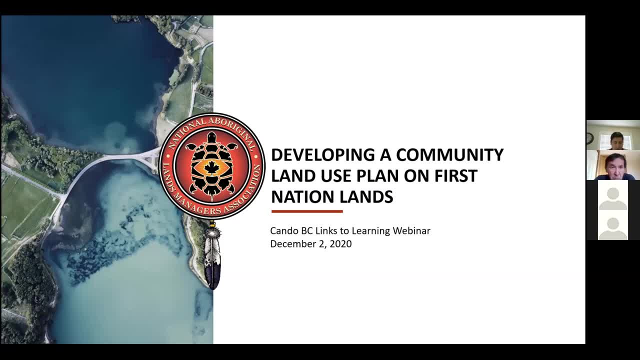 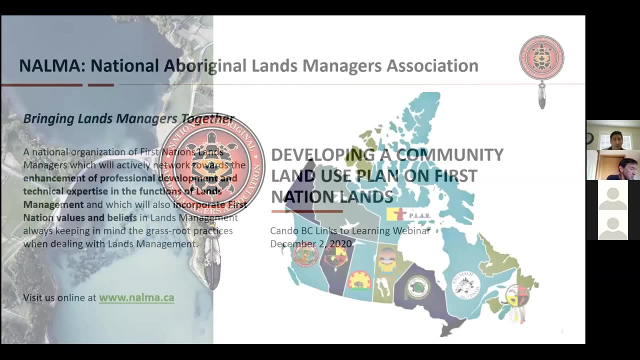 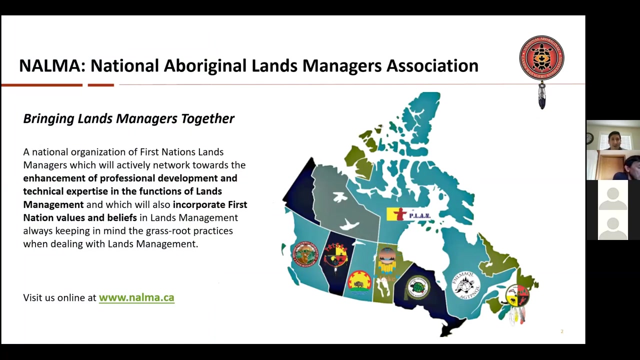 give a thank you out to CANDU for hosting the webinar here today and, you know, further invitation for me to provide this presentation workshop. Thank you, Thank you. Thank you, James, Thank you, Thank you For those in the audience out there that may not know about NELMA- and there's also many. 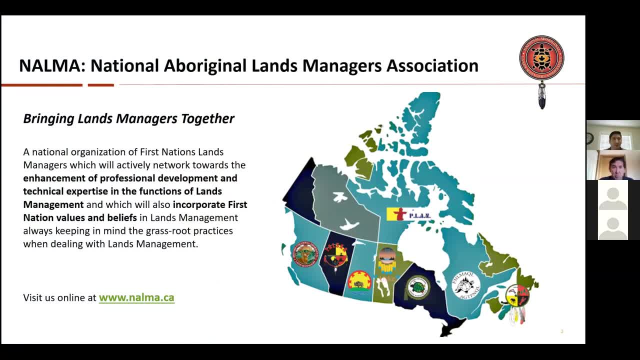 that are. I just want to give a quick little snapshot here just what NELMA is. where I work, The National Aboriginal Lands Managers Association brings lands managers together. It's better known as NELMA, often referred to, And we're a grassroots, not for profit organization of. 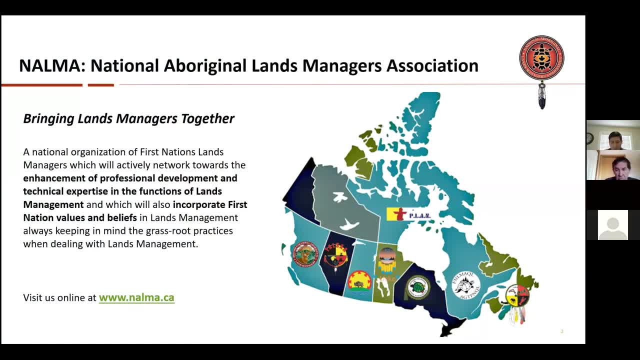 First Nation lands managers across Canada that network towards the enhancement of professional development and technical expertise in all functions of lands management. Also, it's important in our work that we include those First Nation values and beliefs in our systems And we also have several regional lands associations. 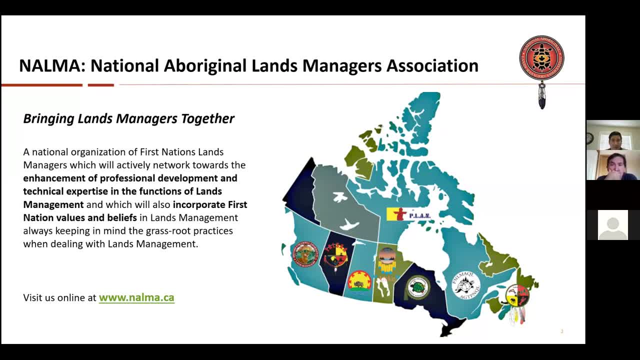 across Canada under our umbrella, For example BCOM in the British Columbia chapters under our umbrella. And for those that are in other regions of Canada, you could look at your regional umbrella organization for land managers. You could check us out at nalmaca as well. 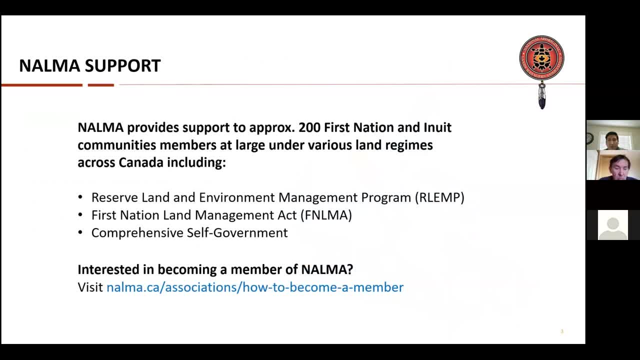 So NALMA provides support to approximately a little over 200 First Nation and Inuit communities across Canada under various land regimes. Three of the regimes you have are LAMP, which is the Reserve Land Environmental Management Program. You have the First Nation Lands Management Act. 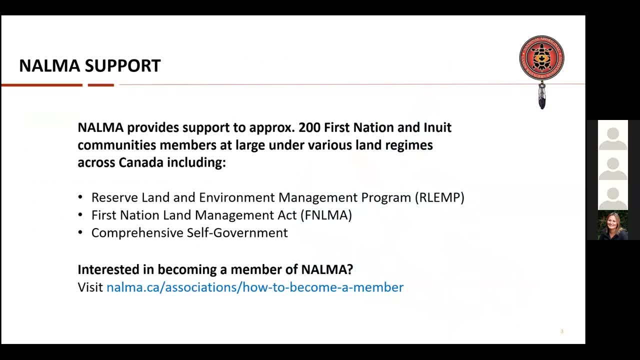 And then you have comprehensive self-government. Some of the land use planning processes may differ between each of these land regimes. Five key functions of our LAMP are often community-based land use planning, lands management, natural resource management, environmental management and 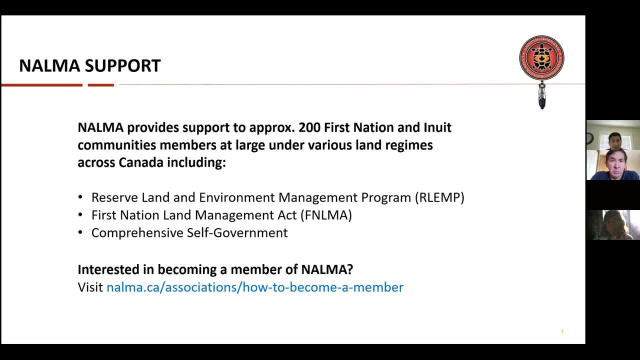 RECONCILIATION, LAND USE PLANNING BASED ON THE BASIC STOREMAKERS PROGRAMS EQUIPMENTED BY PAYAP AND ALSO READY FOR SUPPORT BY PAYAP, AND THOSE ARE ALL BASED ON THE SETTING WE HAVE. 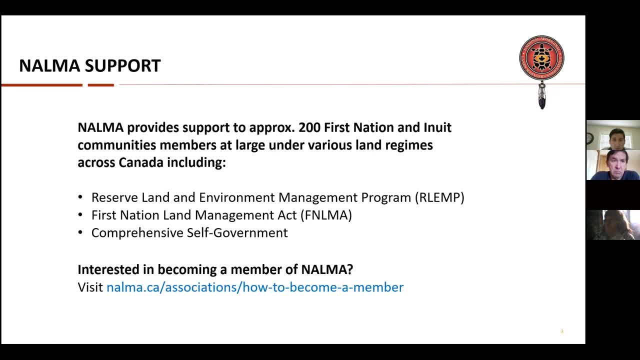 ALSO BASED ON THE EQUITY AND SUPPORT PROGRAMS THAT WILL BE USED AT THE LAND USE PLANNING, SO THEY WILL BE AVAILABLE FOR USED IN THIS AND THEN. WE OFFER LAND USE PLANNING AND LAND USE PLANNING CLIENTS AND LAND PAYBENTS. 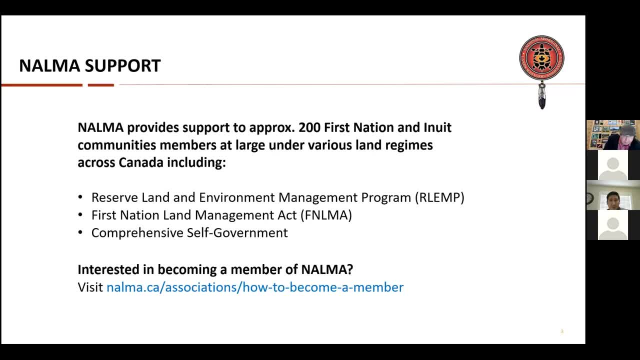 TO BE HELD AT THE LAND USE PLANNING. AND THEN WE ALSO HAVE TO DO PRACTICE: communities at large under various land regimes, reserve land, environmental management program, first nation lands management act and conference of self-government- five key functions of our lamb- i'm just repeating myself just because i was muted there- our community-based land use planning lands. 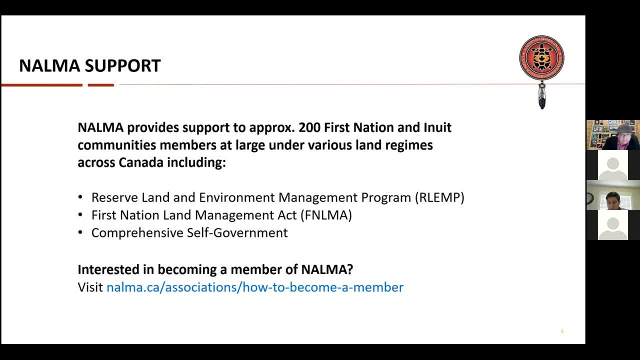 management, natural resources management, environmental management and compliance management related to promotion and monitoring of enforcement on the lands. fnlm is a sectoral self-government initiative to enter first nation lands management. often the first nation will sign a framework agreement with canada. once that framework agreement has been signed by the. 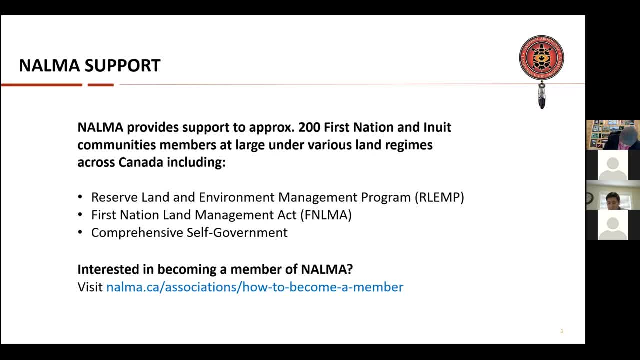 first nation in canada. the first nation will develop its land code, enter into an individual transfer agreement with canada and then, in this comprehensive self-government agreement, set out an arrangement for aboriginal groups to govern their internal affairs and assume greater responsibility and control over the decision making that affects their communities. 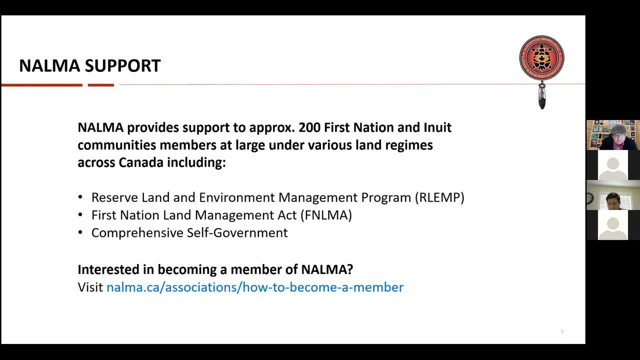 more detailed information on these three types can be found at if you just go to nelma's website, nelmaca, or you can go to labrcca under the first nation lands management resource center. you can also just look at canadaca and search the indigenous services canada or crown relations sections of their 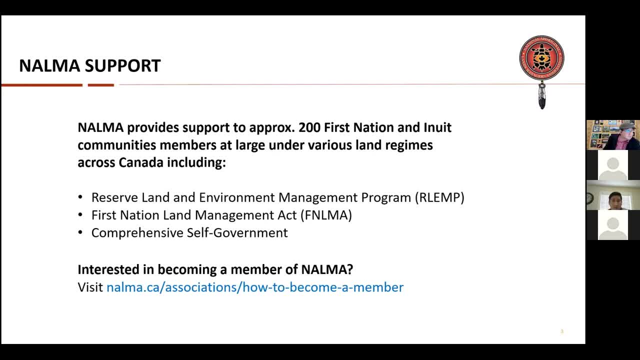 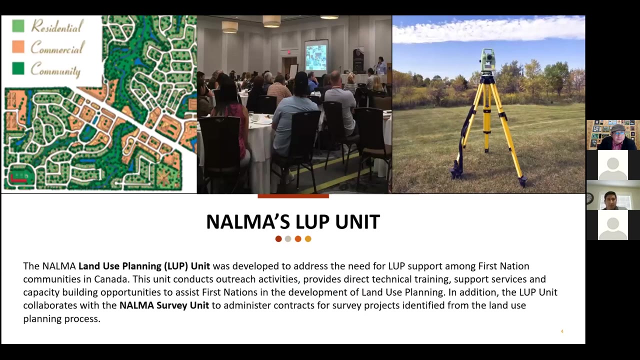 website also for those first nations interested in becoming a nelma association member. you can visit our local website as well and there's information under the local associations link. the land use planning unit here was developed to address the need for land use planning support among first nation communities across canada. some of the things that we do at the lep unit here is: 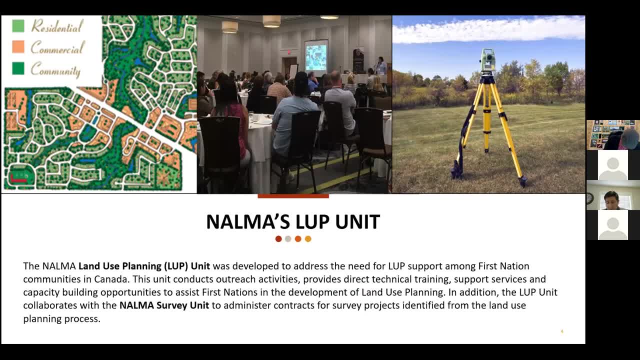 offer outreach activities, direct technical training and support services and it's building upon that first nation capacity and opportunities with land managers. also talk often with economic development officers or land manage or environmental management officers as well. the land use planning, infrastructure and so forth will be brought into the opp 400s community. 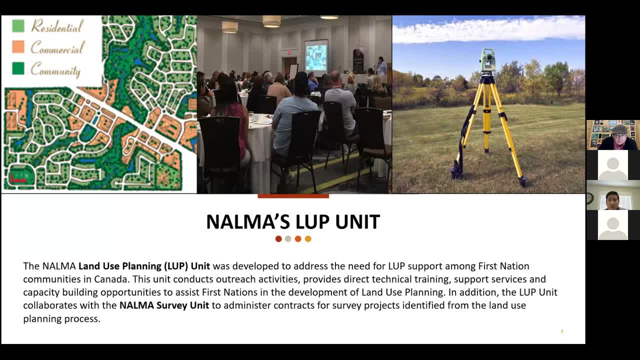 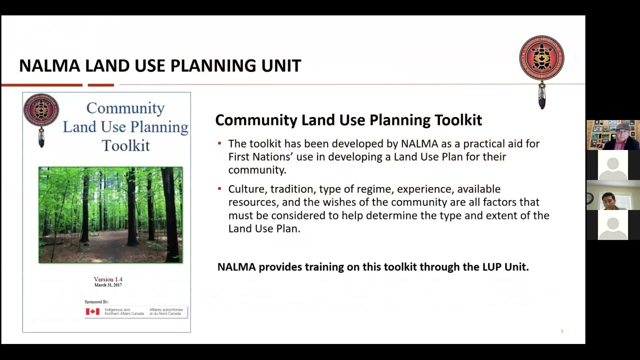 around the land use planning unit to develop and develop and expand these facilities and work that way and also bring in new individuals to the community so we can build a new organization. um, i'm going to introduce myself as a service manager. boundary of the greater First Nation boundary lines as a couple of examples. 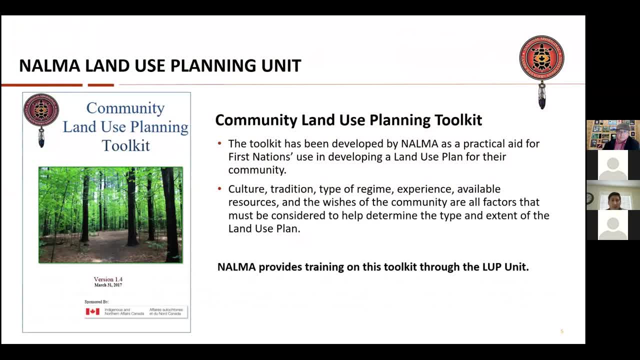 A good guiding book that Nelma has here is the Community Land Use Planning Toolkit. One of the last several years we've provided training in relation to the Community Land Use Planning Toolkit in a number of training workshops. The goal of this part of the program was to build capacity to those First Nation land 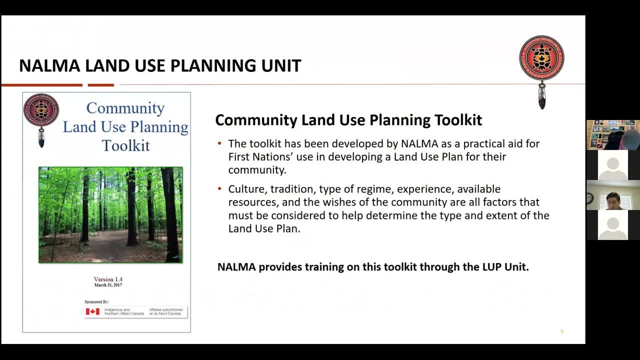 managers that are undertaking and wanting to know more about land use planning This year. due to COVID-19 pandemic situation, we're currently working on providing and switching to provide additional online tools and webinars here locally at Nelma. So we're revamping a lot of our programming to give an online to some of the work that 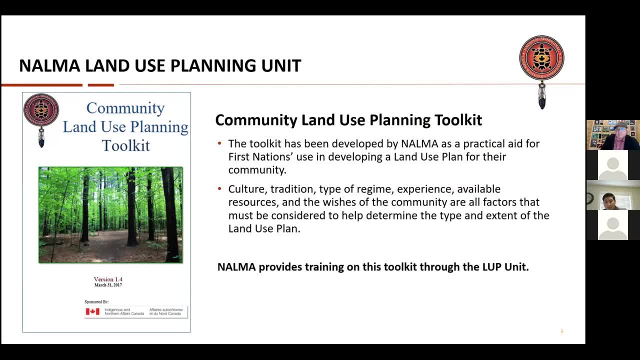 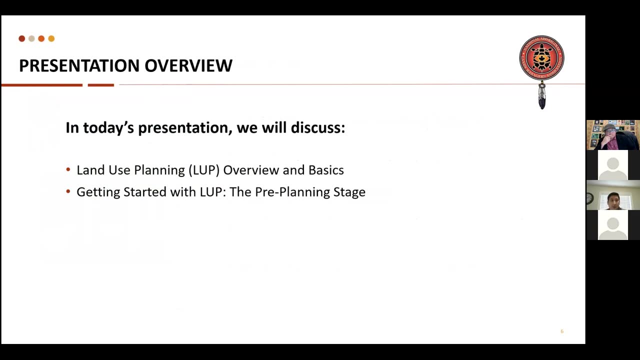 we've been doing In person in many of the regions of Canada. So stay tuned for a lot of those changes that will be coming up throughout the year here at Nelma. So the presentation overview: we're going to be talking about overview and basics of 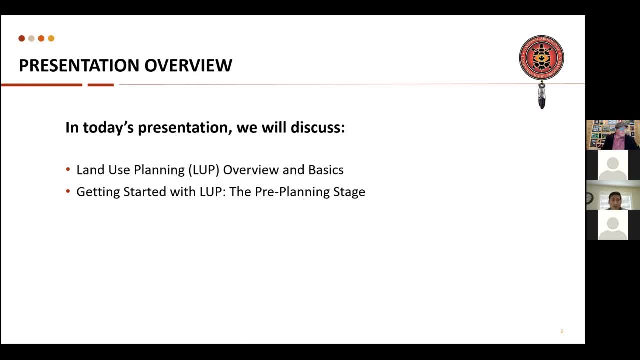 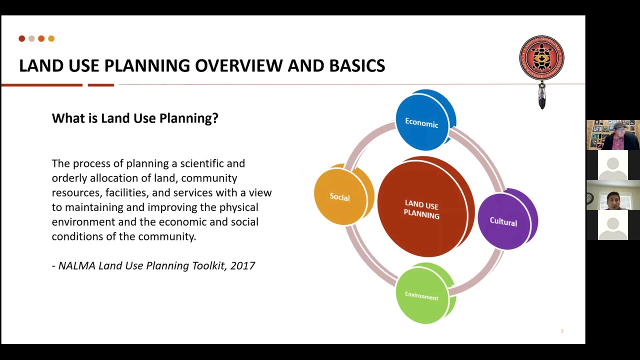 land use planning as well, as often I get asked a lot of the questions is: where do I start? so we're going to talk about starting the land use planning in that beginning pre planning stage of undertaking a land use plan. So one of the first questions overall: 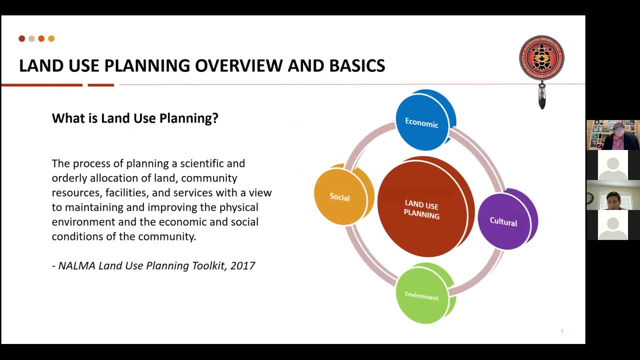 What is a land use plan? I often get asked that question. why do I have to do a land use plan? How does it apply to my specific community? so often, the process of planning a scientific, an orderly allocation of land, community resources, your community facilities or community services, 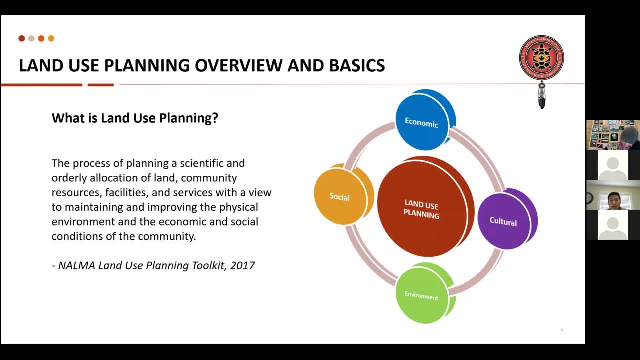 with a view to maintain and improve the physical environment, Also the economic and social conditions of your First Nation community, And so with a diagram here you'll see how land use planning often touches upon all aspects at the administration and community level, bringing in social aspects, cultural aspects, 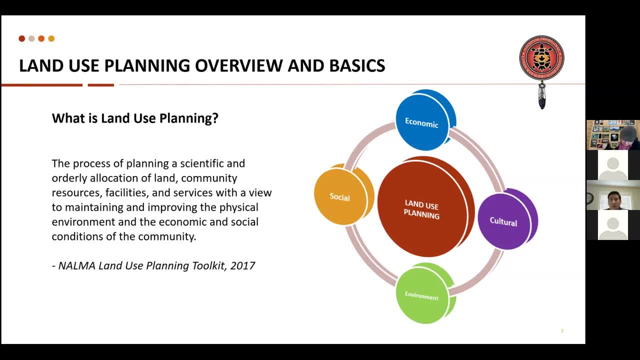 environmental aspects and economic aspects All tie into how we use the land and what we put on the land and where we're going forward in a community. and how does planning overall balance these interests- individual interest of the community members, overall First Nation interests- with those wider interests and objectives? 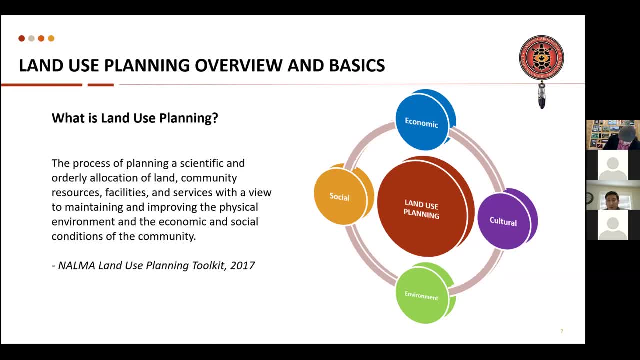 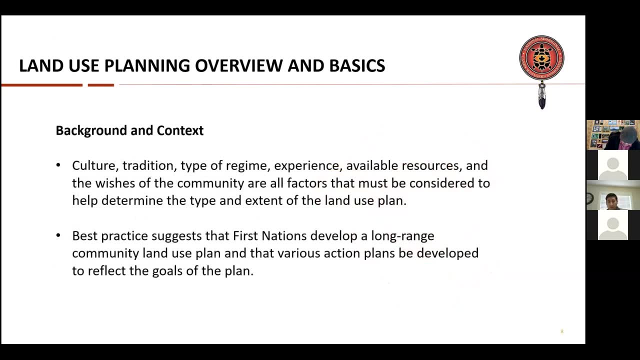 of where the First Nation wants to see itself go as a community and grow as a. as a First Nation community, A little bit of the land use planning background, often your culture at your local community area, as well as the traditions, types of land regime that you may be under experience and. 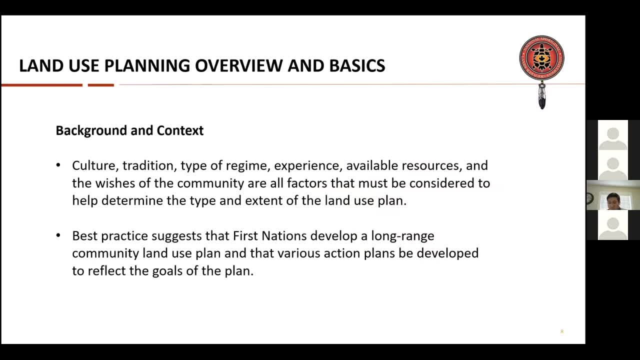 available resources overall, you know what is the community like to see. what were they wishing to see are all factors that would be considered to help determine the type and extent of your community's land use plan. It's also very important to practice and have some best practices and suggestions that the 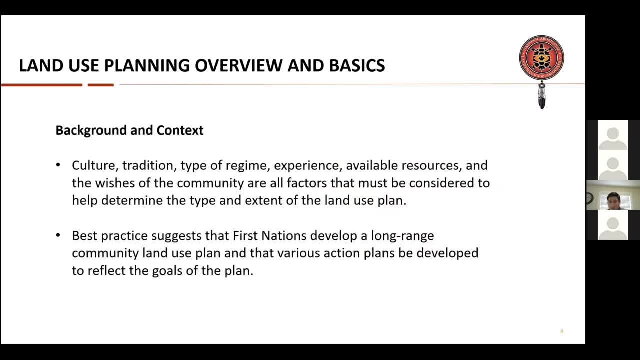 First Nation will develop in this long range community land use plan and it varies depending on the action plan to be developed, which will be reflective of your individual goals at the First Nation level of where you would like to to see yourself go into the future. 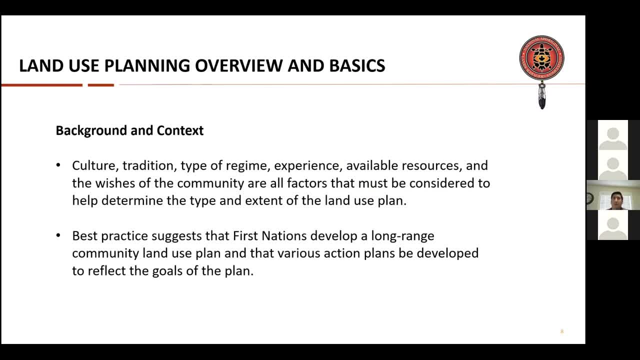 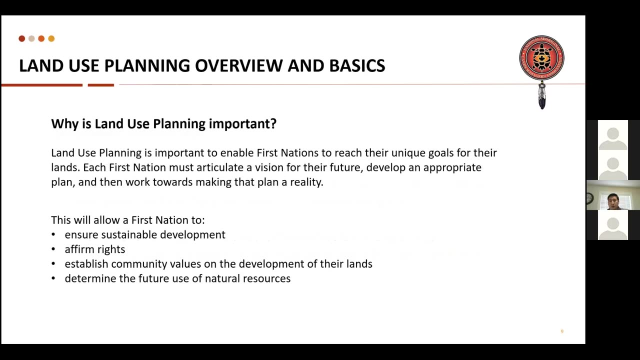 So one of the things with planning is it's not short sighted, it's not about just tomorrow, it's the long range of where do we see ourselves- 1020 years, often down the road- and how are we going to going to get there, to achieve those goals at the community level? 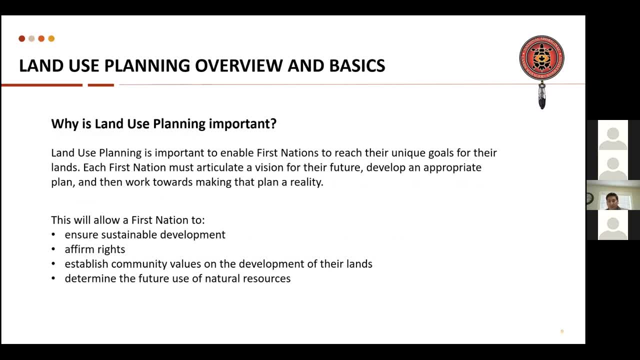 And then one in the next question that often this comes in brings us into is, overall, the importance of planning. Why is it even important to plan so often? LEP is important to enable Your local First Nation to reach those unique goals for their lands. 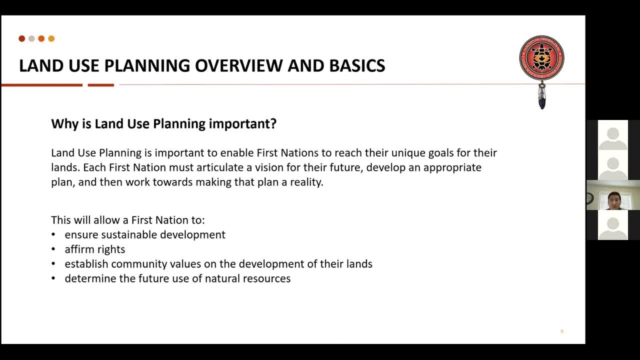 Each First Nation will articulate a vision for their future, develop that appropriate plan and then build upon and have those incremental steps towards making that plan a reality. This will often allow the First Nation to ensure sustainable development is happening and taking place at the First Nation lands and also often it affirms their rights and 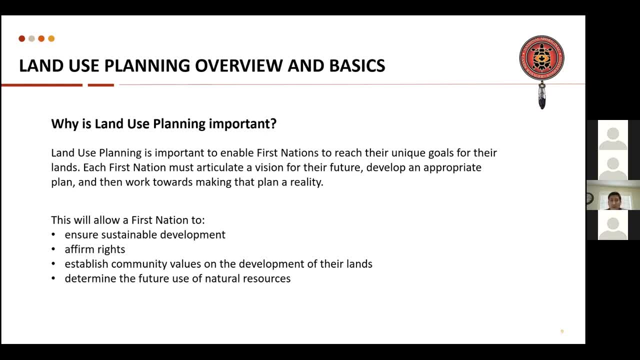 jurisdiction on those lands, Establishing community values in the development of their lands. what do they want to see for economic opportunities to take place on those lands and determining the future use? often many industries- natural resources could be forestry or mining, oil and gas, all depending. 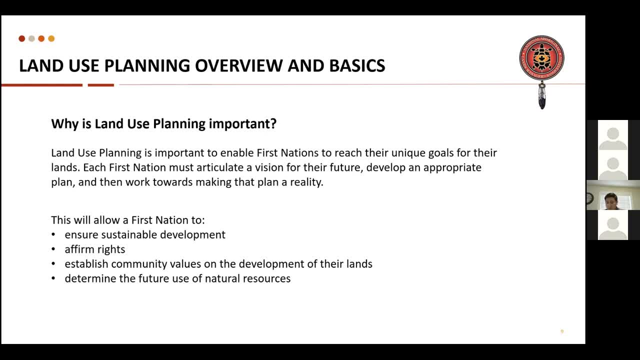 upon your location of what's on your community lands, but it's important to identify, identify these in your lands. Overall, LEP is important to to have the First Nation have a greater say in order to reach those goals and objectives on their lands. 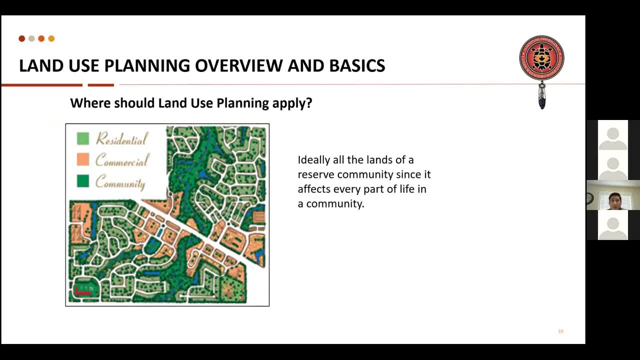 Where should land use planning apply? ideally on all your reserve lands of the community, since it will affect every part of community community life. so your First Nation land use plan would include such areas, as you know where's the current and future: residential lands, Commercial development, industrial areas, agricultural lands areas, recreational uses. 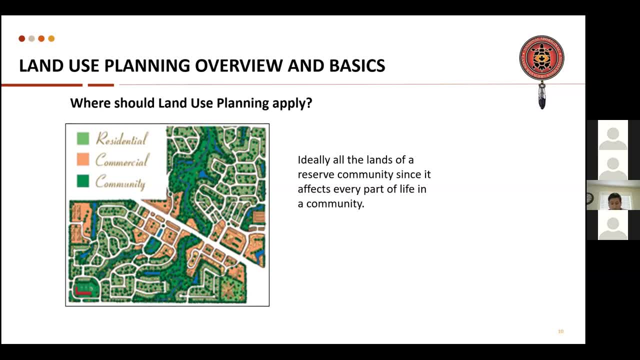 is there any environmental sensitive areas? if so, where are those? Should they be protected? Is there any cultural significant lands that you don't want to be developed and you want to protect those into the future? These are a couple of examples of what to look for when you are doing your local planning. 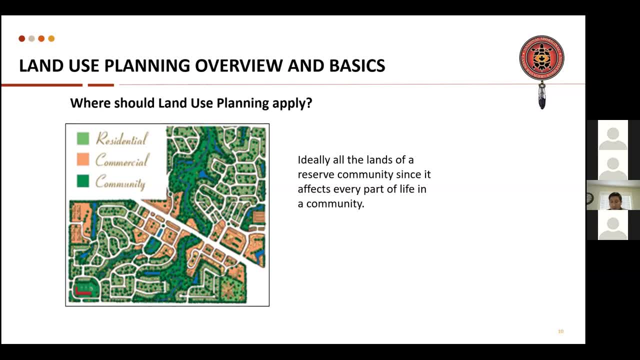 I'm going to turn it back over to you, Thank you, Thank you. Thank you so much, Catherine. Okay, so I will just move over to you in just a few minutes, because I have to continue to talk about some of the stuff that you can get out of your own community land use plan. 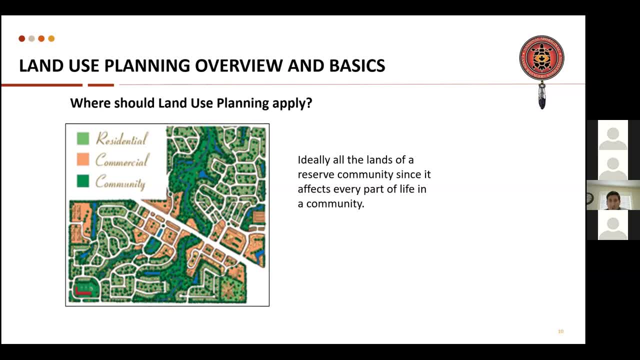 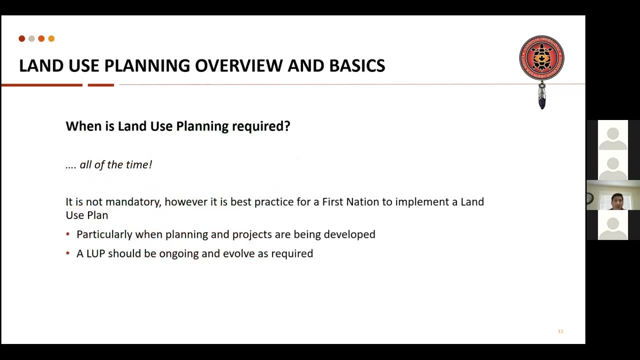 And as you go through the whole planning process you will be able to identify- you know- different instances or unique circumstances as you go through the project. So when is planning and land use planning required? Like to say all of the time. The other question often we'll get is: hey, is this mandatory? 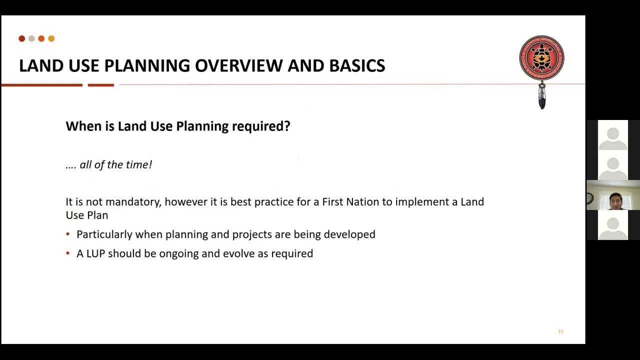 some cases it's not mandatory, but it is very important as a best practice for a First Nation to implement a land use plan, particularly when your planning and projects are being developed at the community, and your land use plan should be ongoing and evolve as required. often, more and more First Nations, you know. 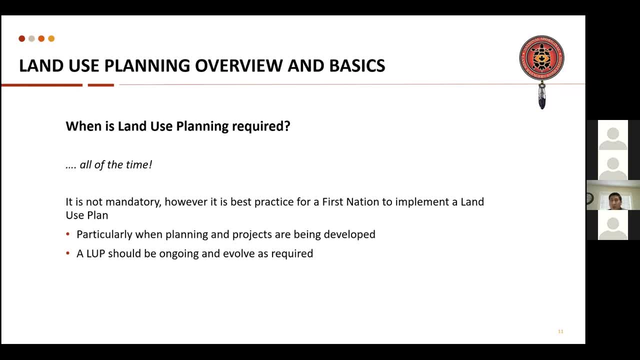 some of them will identify: hey, we have a housing shortage. we need to provide good access of housing types and land tenure. so they'll have a land use plan to identify where is a suitable area for a plan of subdivision. as an example to go, what types of housing is needed: single-family homes or row housing, or 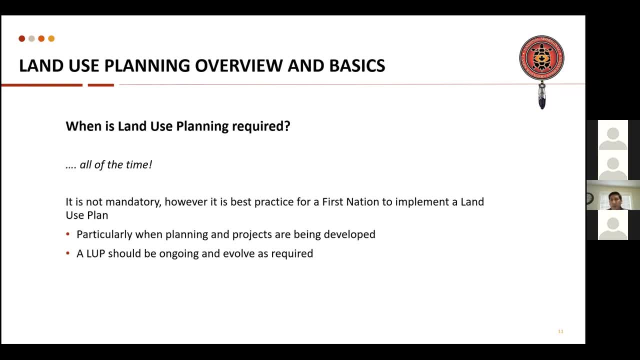 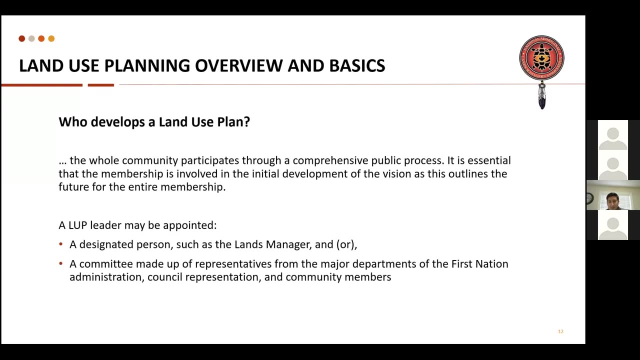 elders or assisted living, types of housing units and a lot of this will come out in planning. as an example, who develops the land use plan? as the next question, and the whole community should participate in part of the land use planning process. it's very important through a comprehensive public process. often this will take place previous to. 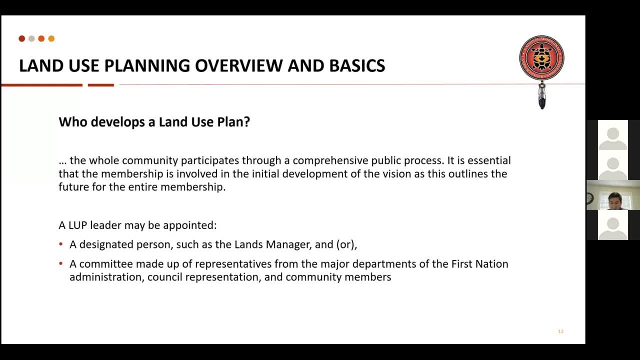 the pandemic, many communities would have a large open house gathering sessions, information sessions or community feasts where they would, you know, if you have a land use plan. it's very important to have a land use plan. talk about the land use plan process and what it entails and get that public. 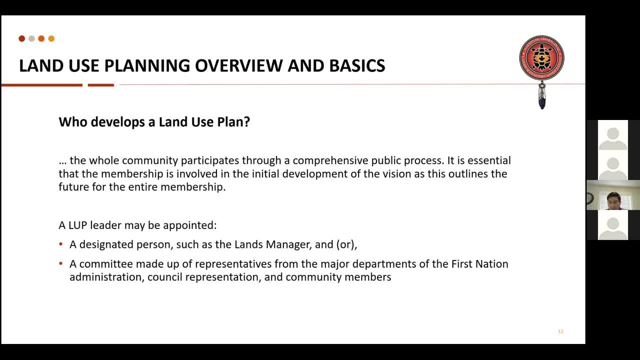 input through those community house sessions. other instances, you know, to continue on with the land use planning work during the current pandemic state that we are in, many communities will now be adopting and creating other options or other means to to get that public information and often this will be: 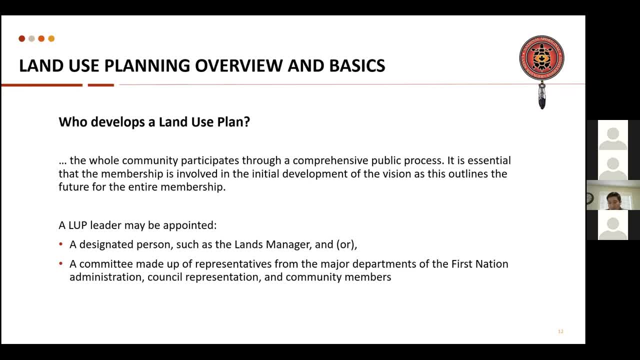 through, you know, virtual platforms like the webinar here today as an example, and you might do that as your community engagement process at your local level. other communities will have online surveys or you can have a mail-in survey. some communities will, you know, have that in person with the staffer and calling various departments. 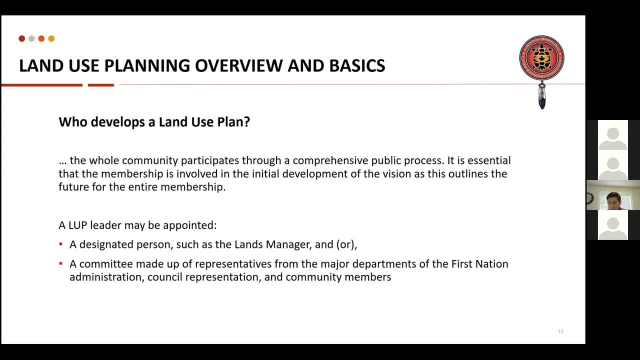 or community members and having a discussion as as non-contact ways to get some of the public input at the community level and continue with that, including the participation level. what's important is uh identifying that land use planning leader who is going to be appointed for the project lead. 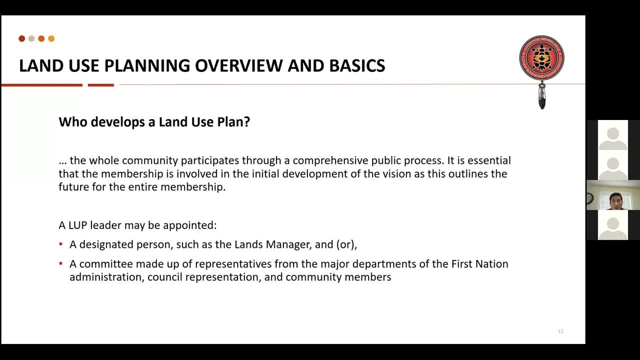 often it's designated, such as a lands manager, or it's an economic development officer or environmental officer. if they don't have a lands manager in their community, often be the project contact lead and often you'll have a land use planning committee made up of representatives from major areas departments at the first nation as local. 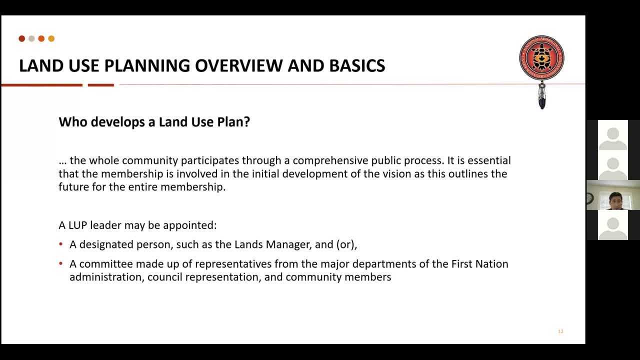 administration and that could be the manager of housing, economic development, social or cultural department areas, education. you can also have a council representation from your chief and council. you don't need all of them, but you could have that council rep. you can also have your community support members. that could be a youth, an elder. other interest areas you can look at how. 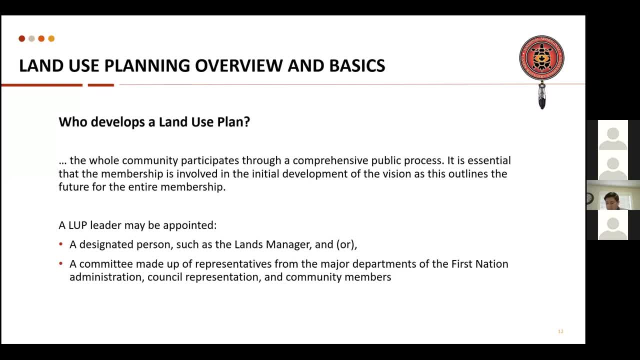 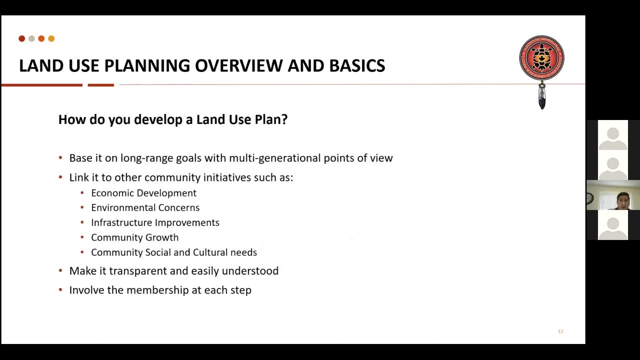 on off reserve are represented at your local community areas for input. these are all baseline examples of of when you're setting up that committee and how you're going to get the information across so often when you're talking about how you're going to start in developing your land use plan. 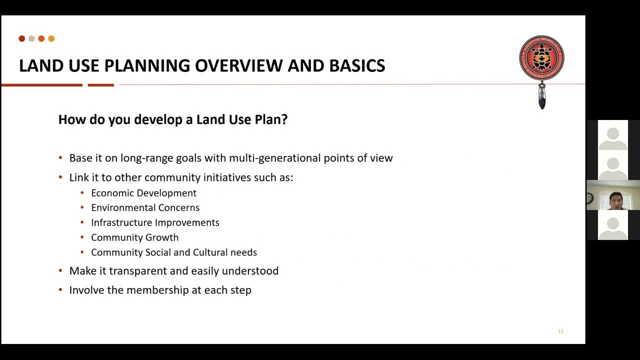 you're going to base it on long-range goals with multi-generational points of view. you're going to link it to other district planning regions based on kennedy's home base already put out. but make sure that you understand and enjoy your area planning plan. it's all up there, all that is. 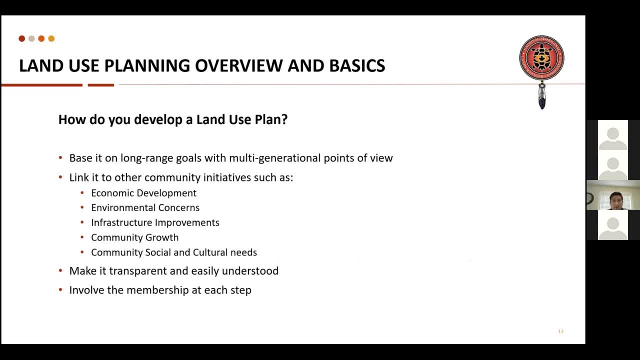 to keep the work you're doing, so it's so relevant for you. also, there's the rip farm development initiative of your project development improvement organization and the project planning capacity. community initiatives, such as economic development initiatives, environmental concerns, infrastructure improvements, community growth and community social and cultural needs. often you're going to make it transparent and easily. 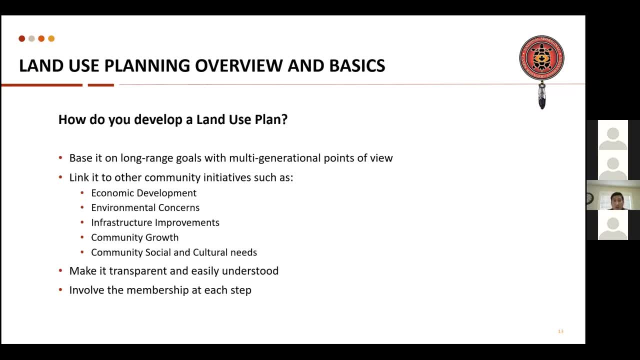 understand document that when you're back at the office you can understand it. as the land manager, economic development officer, environment officer, and and the information that's inputted into the document, you you can easily understand it and read it, and and and move forward. it's also important to involve the 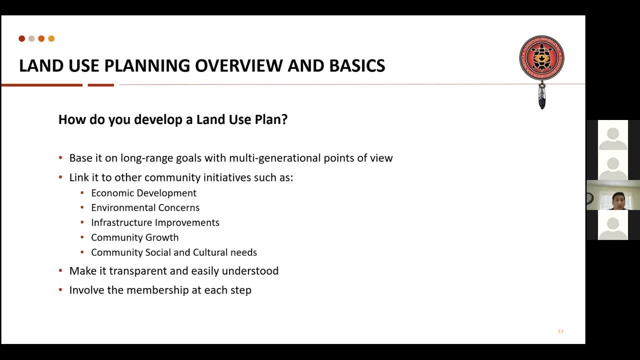 membership at each step in process as you go through the land use planning process by engaging in conversation as well to a lot of these projects. often when I go into different communities, they're doing- they're all busy. they're doing a lot of work and often they're so busy that they forget to to talk. 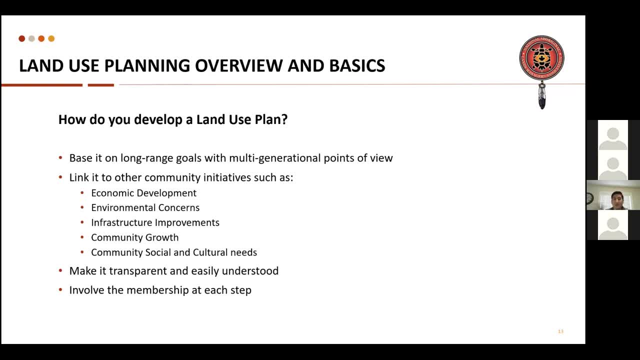 about the land use planning process and they're so busy that they forget to talk with one another in the cross-section of all of their departments. so often economic development has a lot of projects on the go and and they may not have meetings with you know their environment side or the land management. 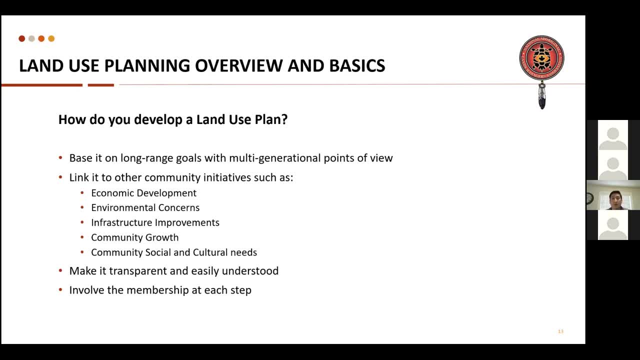 side or other department areas, and it's important to share that knowledge of what everyone is doing and then also taking that, incorporating that as part of this planning process- and you'll start to see different overlap areas of some of the project and who should be involved- and incorporating this into. 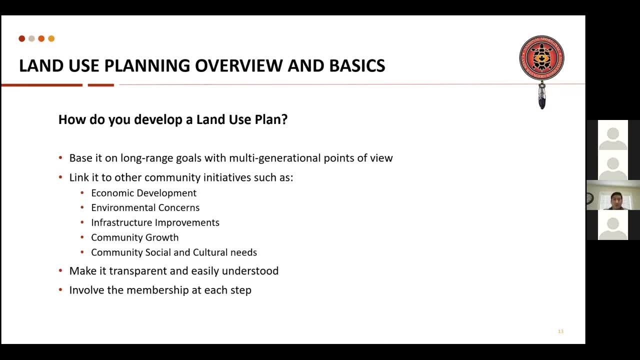 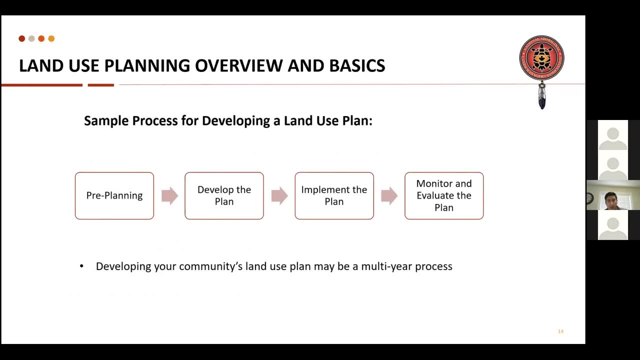 your land use planning and involvement areas in addition to membership. a sample process we have up here of developing a land use plan gets into what we're talking about here today. on on pre-planning: The pre-planning from beginning to end can often take, I see, on average again. 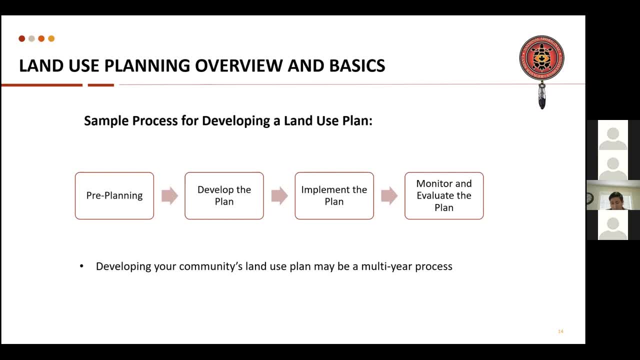 these are all timeline estimates. Actual timelines will vary for each First Nation due to a variety of factors, but the pre-planning can take about six to 12 months And that could just be from the day one where you read and learn about what planning is and how you can start and research. 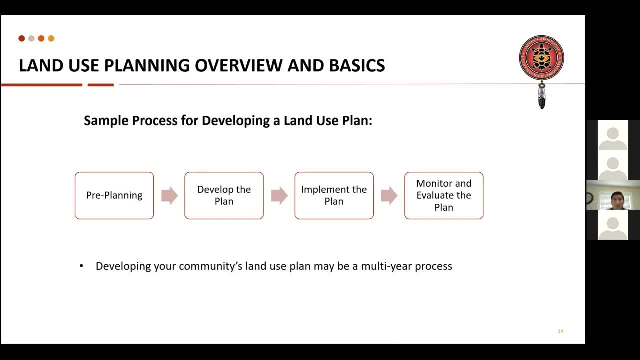 on doing a land use plan in your local community and then presenting data you know with your internal department or your band manager and then bringing that forward into your chief and council area And then you can also start to develop the land use plan And on average that will take. 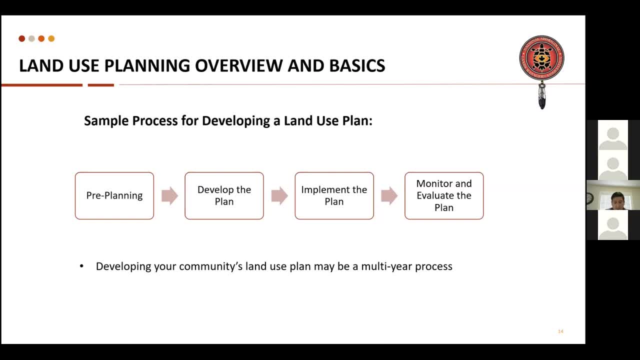 about six to 12 months And that's the real meat and potato Of actually doing the land use plan and getting you know. after you have done all your pre-planning stage, you can start to develop the actual planning process, Implementing the land use plan. 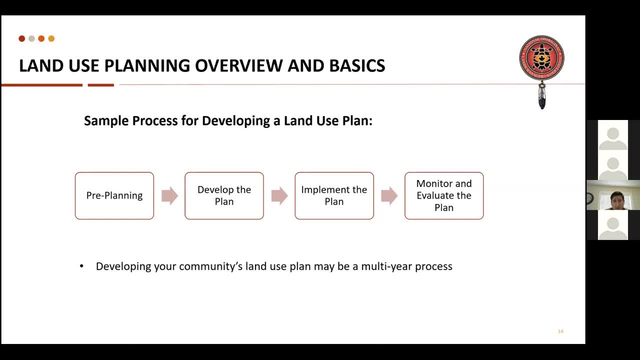 can be about three to six months, And that's we did the pre-planning. we have background information. then we develop the actual land use plan of where we're going for the next 20 years And then how are we going to implement the land use plan? And then how are we going to implement? 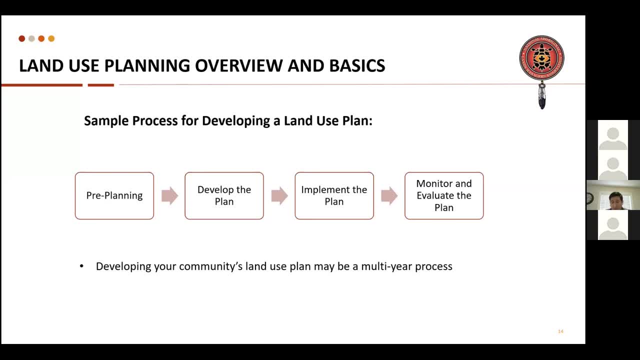 the land use plan And you're going to install that implementation plan of putting the plan into action, into play, And that could be about three to six months. And then you're going to have a monitoring, evaluation of the planning process And you're going to put 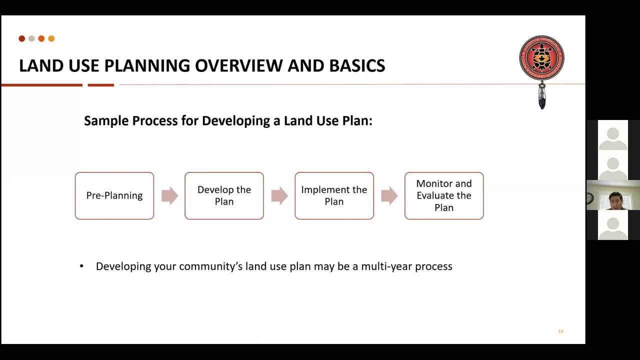 steps of how you're going to monitor, how you're going to evaluate if the plan is working, And so putting the background work into that will take about three to six months on average, But developing your community's land use plan overall is a multi-year process And that's. 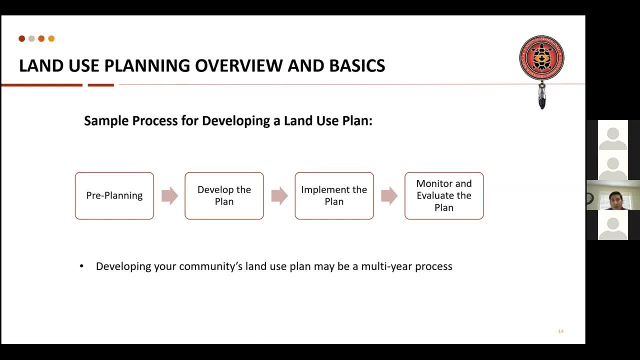 going to take anywhere between one to three years, And that all depends on where the stage of First Nation communities are at. Some of them have very little information and knowledge And they have little bits here and there in text forms. Others have a lot of previous studies that 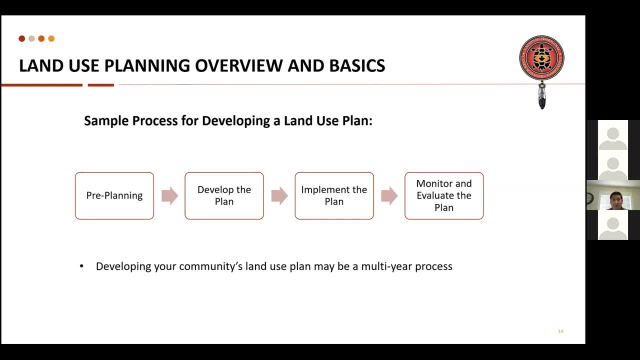 were done, And it's a matter of collecting these studies. say, if it's a capital planning study, if it was an environmental management study, they might have an economic development study, And then you're going to have a lot of information and knowledge, And then you're going. 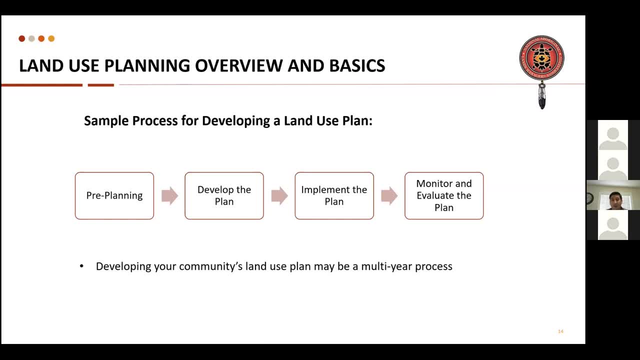 to have a lot of information and knowledge, And then you're going to have a lot of information to plan in place, And so you're kind of gathering, researching a lot of this information And then, before you know it, you're like, hey, we actually have a lot of information. And then what you're 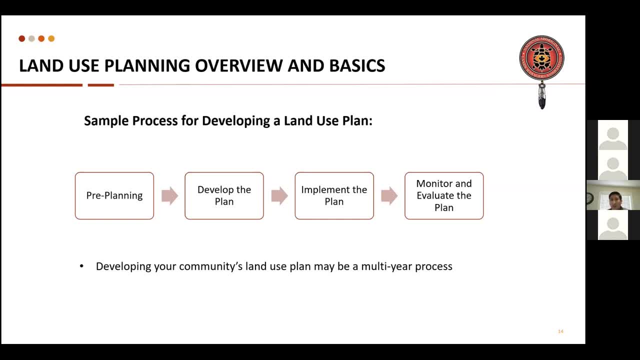 going to do is gather and document that information And then you might look at incorporating different aspects of these different documents as part of your whole land use planning process. So that pre-planning stage is very important at figuring out where your community stands and where you're at and what types of available information, And then you're going to have a lot of 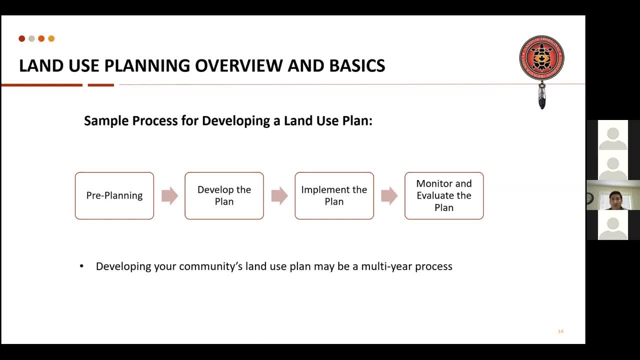 information, And then you're going to have a lot of information, And then you're going to have Antony tenir about what is currently out there that you have, and then filling in the caps of what you are missing as part of your land use plan. 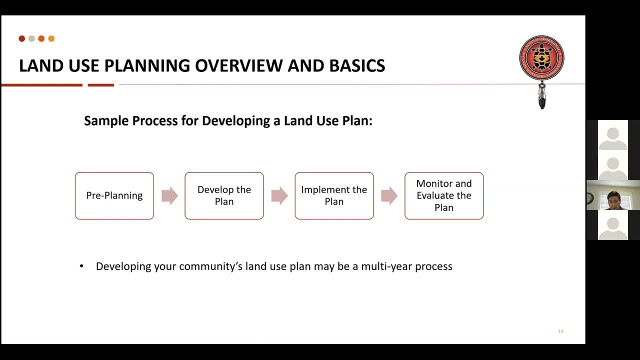 So we have here Arc development phase of talking about a sample job document. Often people reach very simply, who will Вс talking about a sample job document. Often people are like, hey, What does our land use plan look like? Very, very exact. And the Dad who was part of this 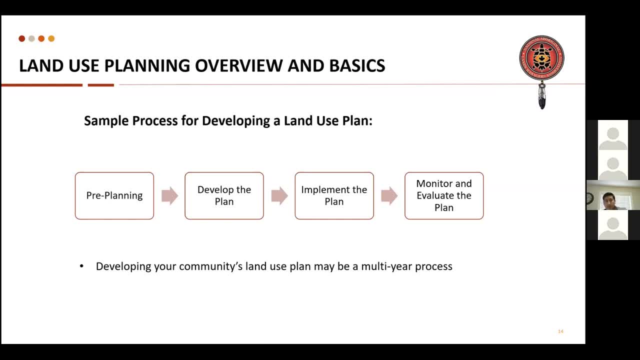 that we brought up. if this really kind of rearranges the course and theань's 10 years down the Well, they're showing now conversations, you know where they have a level of movement in terms of using it, And so what you're seeing is- and I think you have to you- 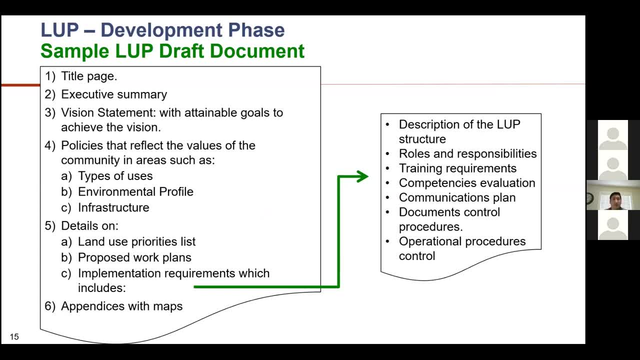 know you have to ask- You're doing the math part of the framework here with expressions development phase- of talking about a sample draft document. often people are like, hey, what is our land use plan? look like very, very example base here. often you'll have a title page. you know Nelma, First Nation. then you're gonna have an 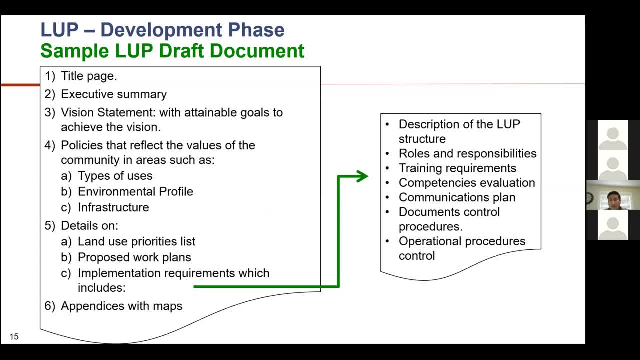 executive summary which is about one to two pages and it just gives a summary of the overall with what's inside of the document. you're gonna have your vision statement at the First Nation level talking about their attainable goals. to achieve that vision at the First Nation level, you're going to have policies that 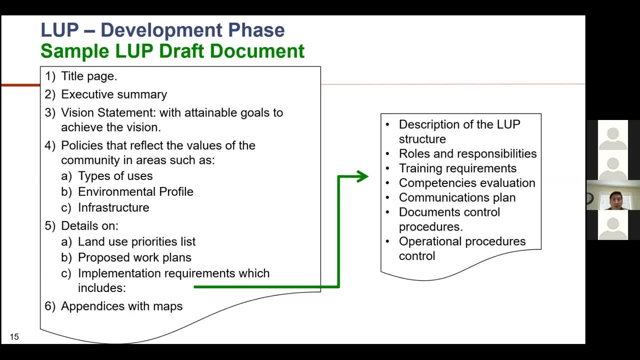 reflect the values of the First Nation community areas, and this can be a variety of areas. one of them would be types of uses of the land, so there could be a variety of uses, from industrial lands, commercial lands, residential lands. commercial lands, commercial lands, residential lands, residential lands, community lands, which can consist of your community. 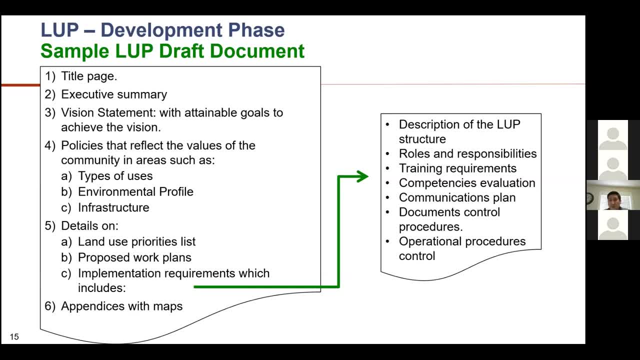 facilities, parks or open spaces, natural lands. natural lands could be hunting lands or natural habitat lands, depending on what's on your land areas. you'll also have an environmental profile on your lands infrastructure, looking at what is your current state of your infrastructure lands this could be is the. 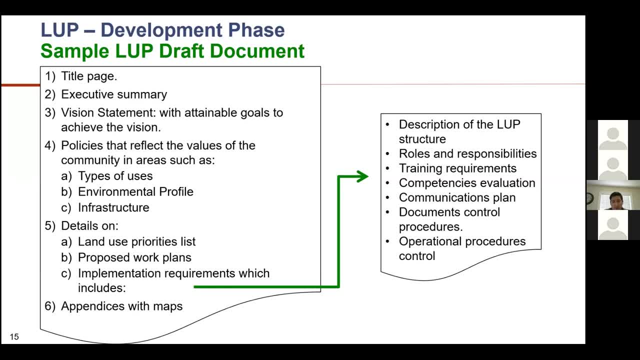 existing infrastructure, roads, conditions. what is the state are they in? is there an expansion for infrastructure that is required or needed? on the First Nation lands details on your land use plan so you could be looking at land use priority list. often there's a identified area of priorities that the First Nation will. 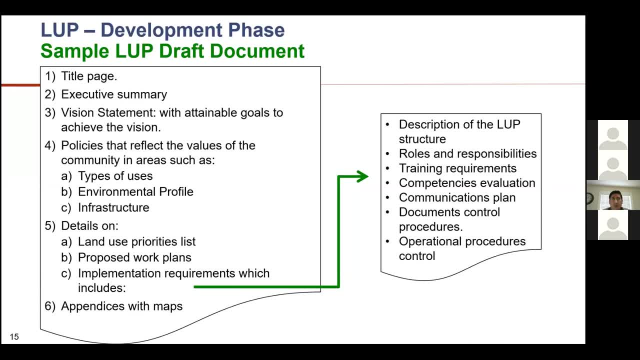 look at a lot of projects or a lot of priorities that the First Nation has and it's a matter of prioritizing them throughout the land use planning process that are identified. so if you're looking at over a 20 year time range, how can you get this work done over that 20 year time period? this is not all going to be. 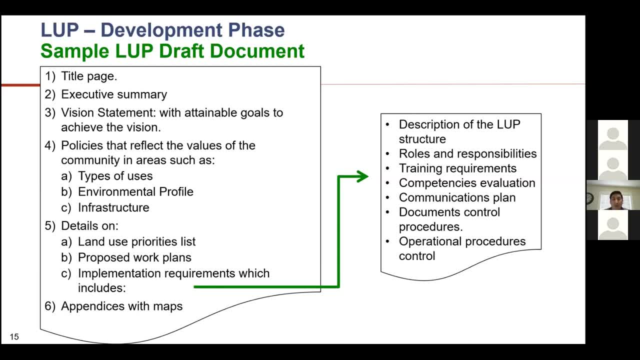 done tomorrow or, okay, over a year. it's going to incrementally be tackled and throughout that process you will achieve your end goal of tackling this priority list. often you might have work plans and other implementation requirements, your implementation part of the plan. often you're going to just have that. 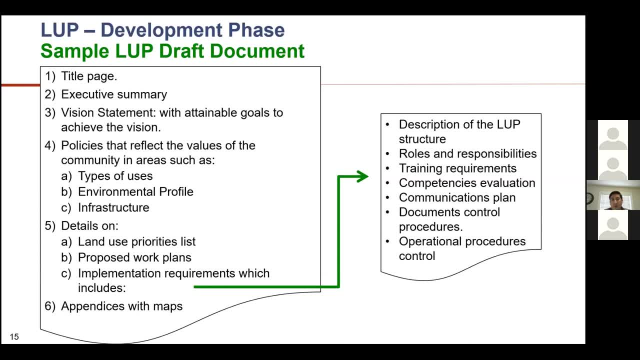 description of your planning structure at your local area, roles and responsibility for different projects, of who's in charge of different projects. sometimes communities will identify training requirements. often, in regards to your land use plan, you'll have laws or bylaws. you'll also have communication plans, document, control procedures or 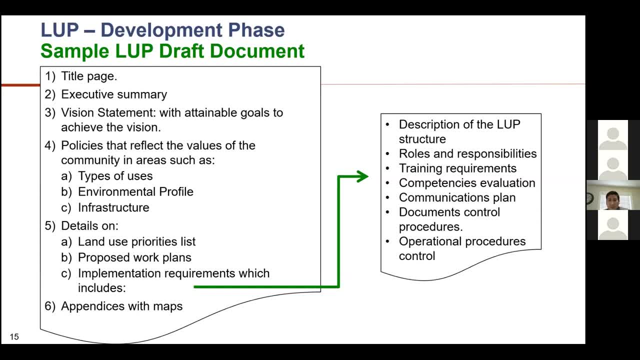 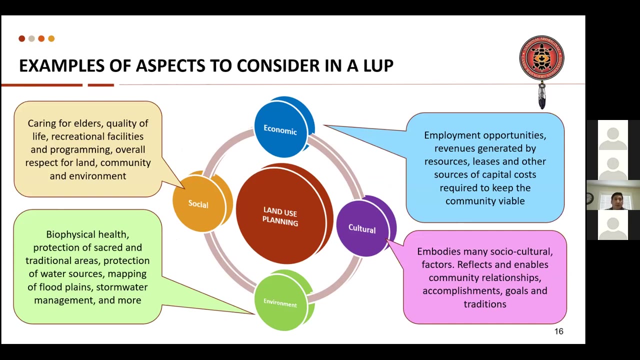 operational control procedures as part of your plan or appendices to your plan. overall, your land use plan will have a land map for your current or future land uses that are part of your land use plan, some examples and aspects to consider overall. just some examples I have posted up here. so if we look at 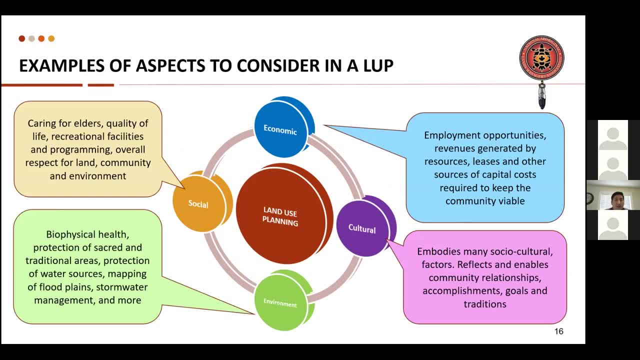 social aspects, often as part of your land use plan, is when one question that always comes up is caring for your elders, providing them with an accessible space. how can that be incorporated into the land use plan? looking at overall communities, quality of life, recreational facilities, you know what types of 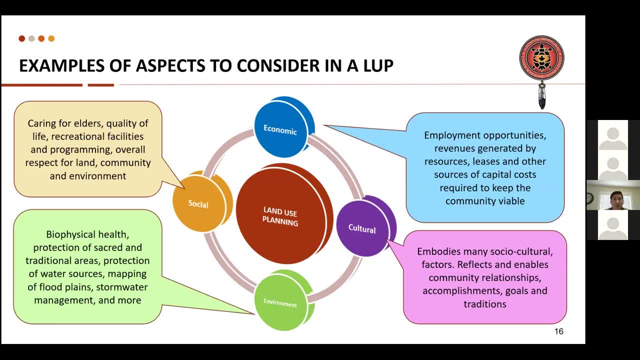 facilities may be needed in the long run at the First Nation, and where can those be located? overall respect for the land, the community environment and some aspects, for that is, you know, creating those laws or bylaws at the community level which will provide some level for, and follow through an enforcement, an environment as well. often they'll talk 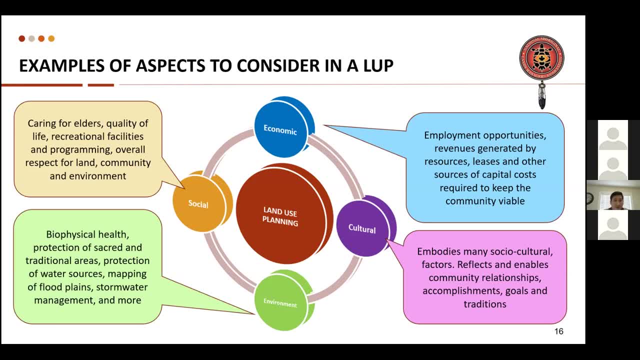 about biophysical health, protection of sacred and traditional land areas. there might also be a need for protection of water sources, sensitive areas, mapping of floodplain. some communities are in a low-lying area and there's, you know, areas where no development should go. other areas as well might require stormwater management. these are all. 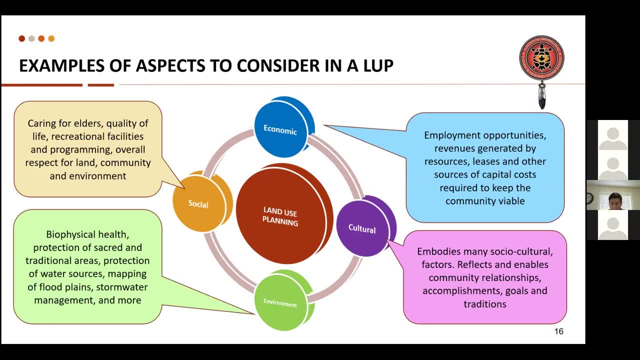 environmentally related matters. there's also cultural areas. this could be, you know, social, cultural factors, having, you know, cultural inclusion and reflect for their community relationship and accomplishments, their goals, their traditions. you know, noting that, noting cultural areas or cultural organizations in general, such as heritage sites and cultural sites. 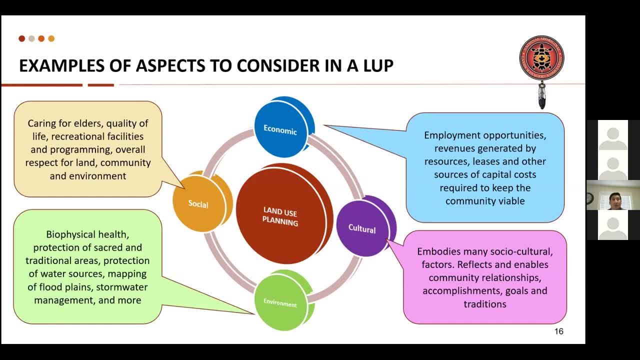 can be protected by land access and which would be the most important part, but these are the areas that are most important to the community that we're talking about. the first, first one, the most important thing, is that you know land use of water in the community, the land use of natural 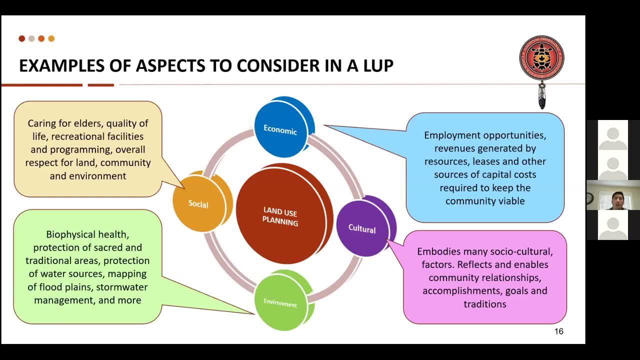 water. the land use of land is not necessarily healthy or bad, but is still important and is a protect and protect the community and the land and the land use are important. a lot of the residents, their families, their employees look at employment opportunities and revenues generated by resources or land leases, other. 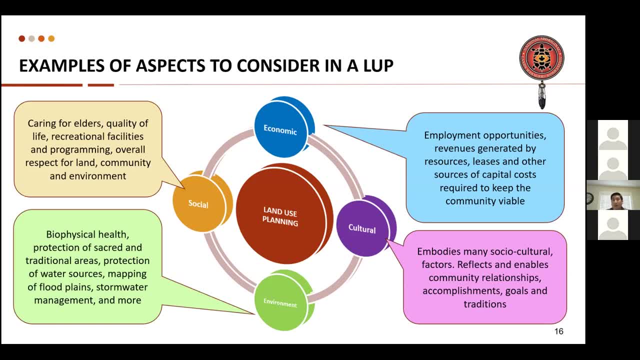 sources of capital costs required to keep, you know, the community viable. how are we going to get an increased employment for, you know, our community members? where can potential businesses go in a commercial area or industrial area, depending on what that type of land use, uh location is. is there a? is there a a highway that runs through and we can, you know, generate? 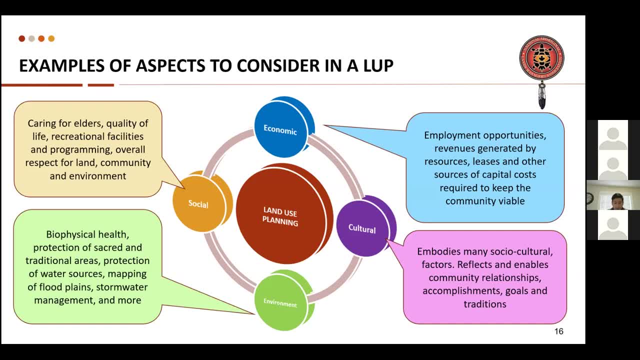 and create economic activity. so it's important to note that the, the land use, needs to combine all of these factors together, which will achieve overall a sustainable approach to to the the very varying needs or competing needs at the community level that they would like to see and include as part of the land use plan. so i'm going to turn it over to the next speaker. 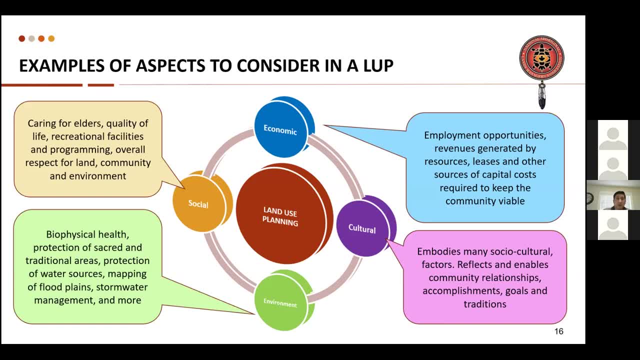 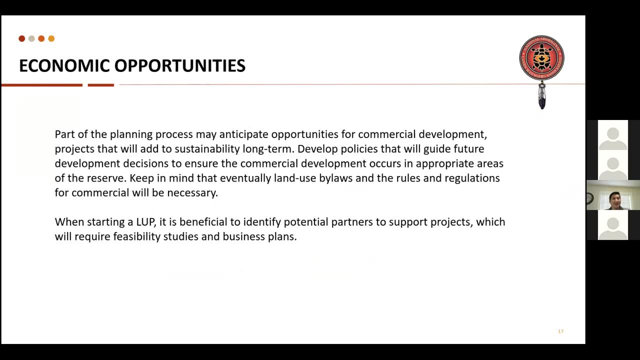 so i'm going to turn it over to the next speaker, land use planning process, because there's a number of of uh economic managers, i believe, on on the call here we would also. this slide is for economic opportunities in a land use planning context of you know part of the. 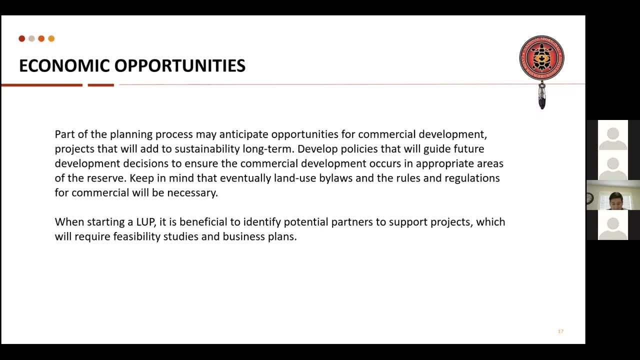 whole planning process may anticipate opportunities for commercial development projects that will add sustainability to the long term. you can also develop land use policies that will guide future development decisions to ensure that commercial development occurs in appropriate areas of your reserve lands, always keeping in mind that eventual land use bylaws or rules and regulations. 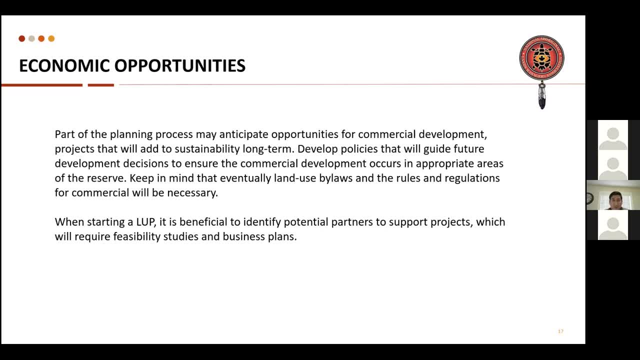 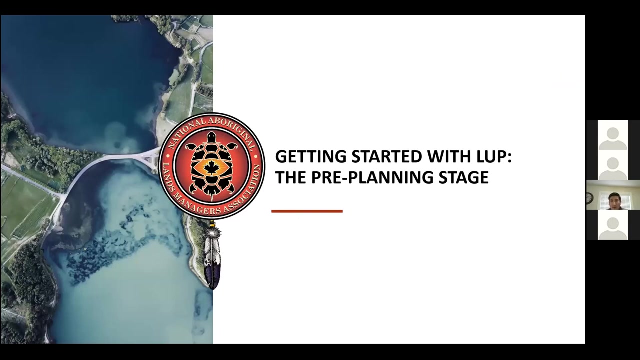 for that commercial activity, depending on what what takes place will be necessary and also when starting your land use planning project. what is the best time and place to start planning for land use and when does it take place? what do you want to do? what can you do? how can you help? 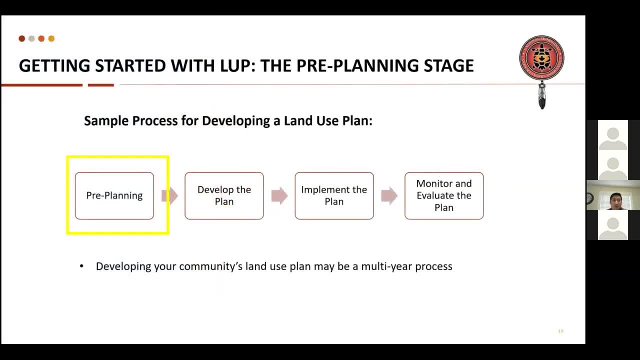 so so my name is isn't my name is a very, really long sample process for developing the land use plan. this next part we're going to talk about the pre planning stage and- and this all ties into the overall community land use planning- how it takes a while as part of that multi-year 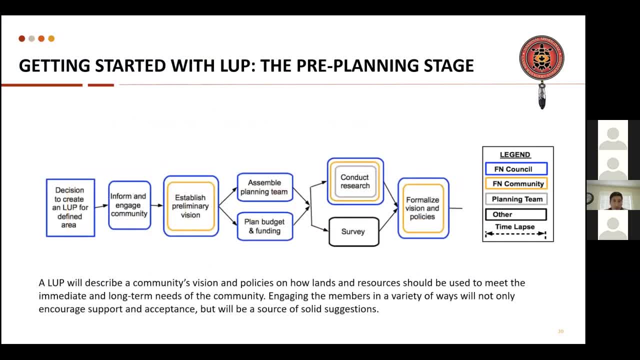 process to complete. so the land use plan will describe a community's vision and policies on how lands and resources are to be used, looking at, you know, short term, immediate needs and then long term needs into the future of the community. engaging communities in a variety of ways is very important, encouraging that. 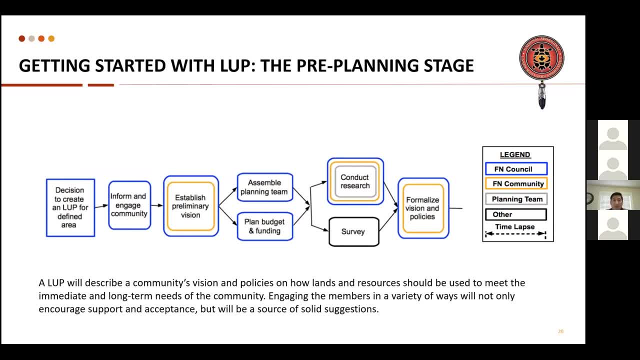 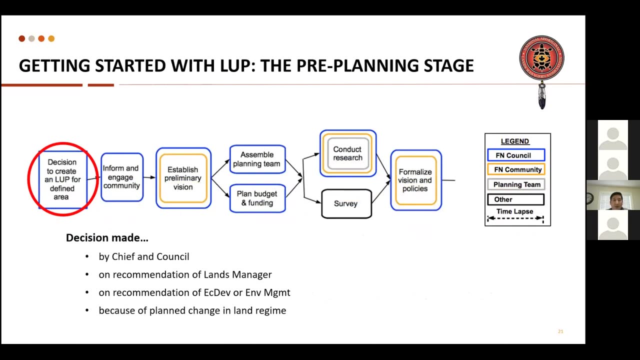 community support. your community buying or acceptance is and and having a number of suggestions. often there's a lot of discussion about land use planning and land use planning starts, you know, that overall decision: hey, I want to do a land use plan in the community and so you'll have. the council often will have a decision that you know. 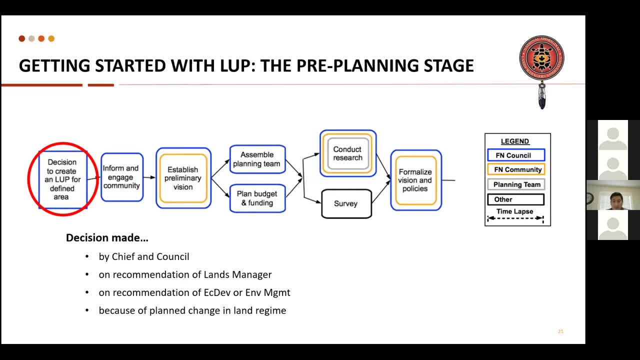 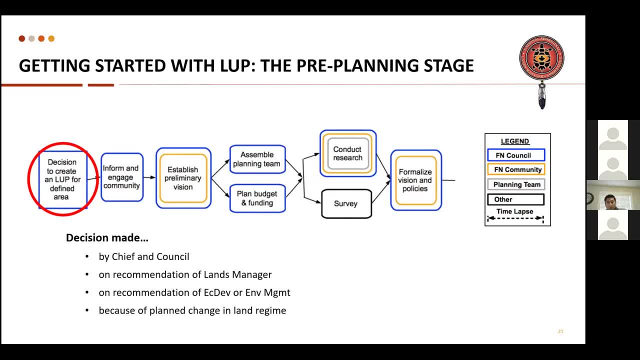 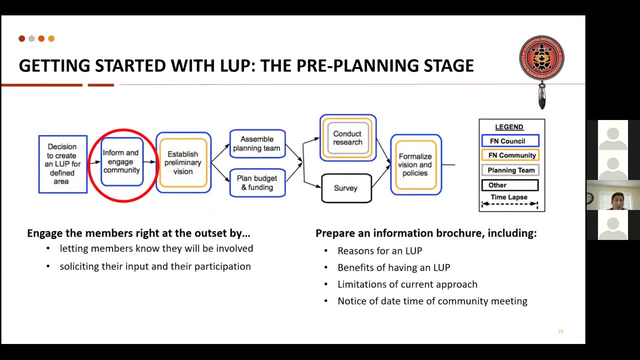 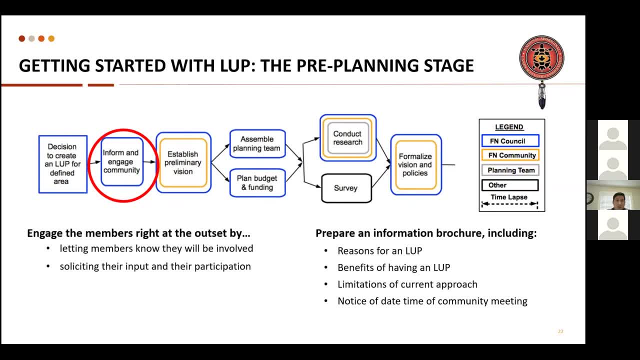 the community, and so you like to engage and inform your communities on the very beginning, letting the community members know that you're going to involve them, them throughout the process. you're going to be, you know, asking for their input and their participation. you can also have different information done up in advance and included. 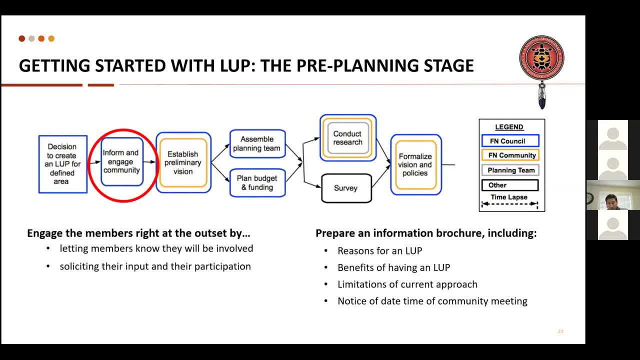 in a brochure- and this can be very simply one page- just giving them a reason why you're doing the land use plan. what are the overall benefits of having your land use plan? one of the things is also setting your limitations of your approach. so when you do your land use plan, for instance, it 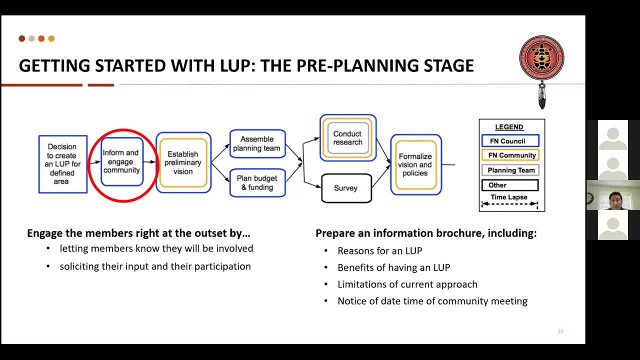 would be focused on your, your current land, reserve lands, as a next step or a next project. you can, if if get asked about the traditional lands or the treaty area, you want to set the stage for the scope in the focus area, because these are often questions that that get brought up. 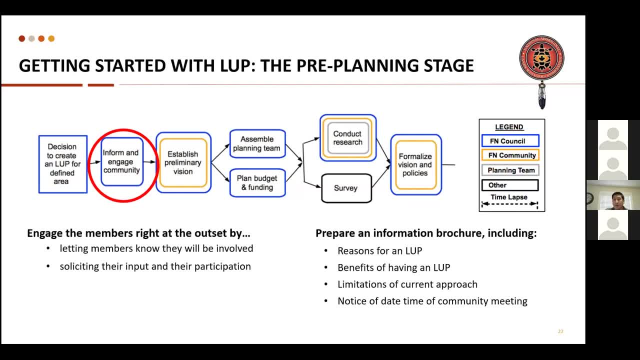 you're also going to have a notice or a with dates of your community events. so when you have engaging for event or input, you want to get get the community information out there in advance of what these dates are. you don't want to just, you know, send a news, a news feed, blurb that you're 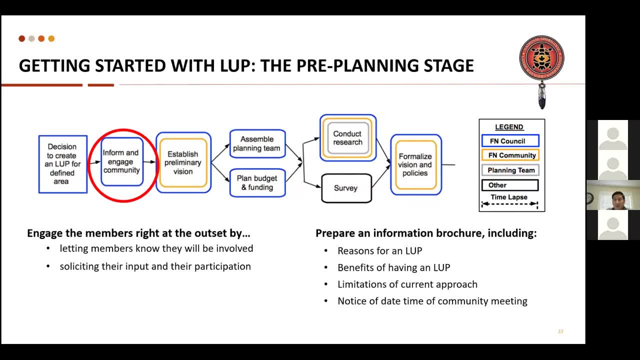 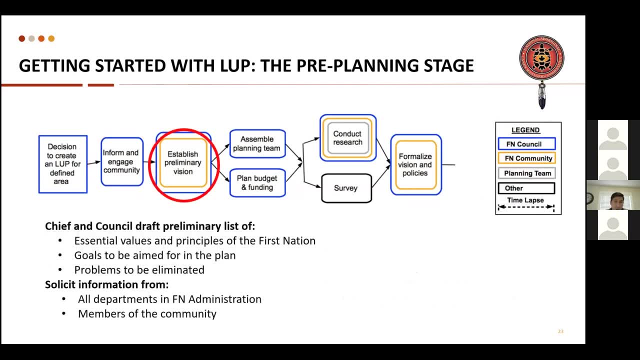 gonna engage them tomorrow and then that doesn't give them time to prepare or make time to participate, so you'd like to do that in advance. establishing your preliminary vision is important, so your chief and counsel will draft a preliminary list. often it's, you know, considered your essential values and principles of the First Nation. what 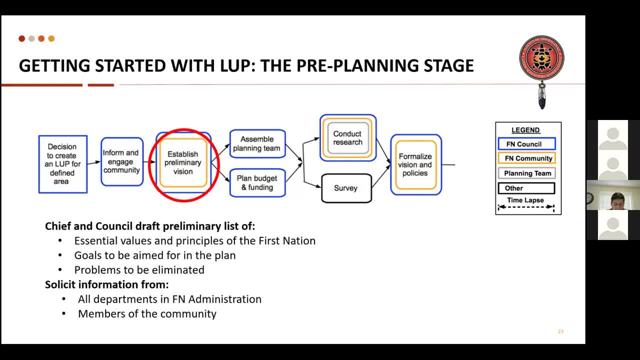 are the overall goals to be aimed for in the land-use plan. you can often identify problems that you would like to be tackled or eliminate through the land use planning process. often you're going to get and ask information from other department areas at the First Nation administration. so the land manager 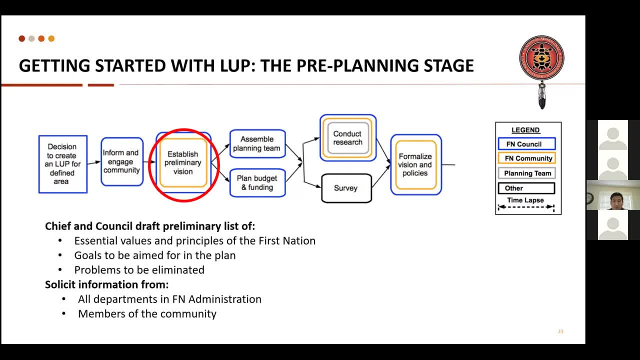 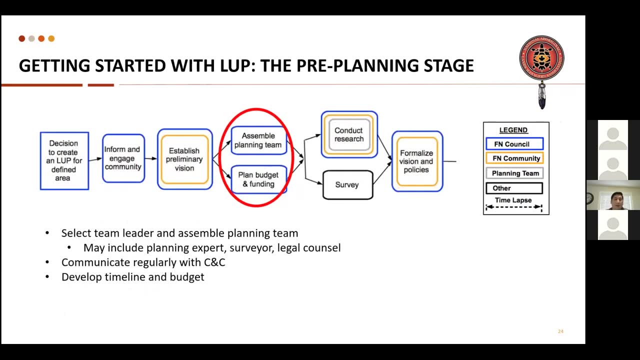 economic development. whoever is in charge of the land use planning project will often be in contact with other First Nation area departments, and then you are also going to be contacting and talking with members of your local community. what's also important is assembling your planning team, and so often this is. 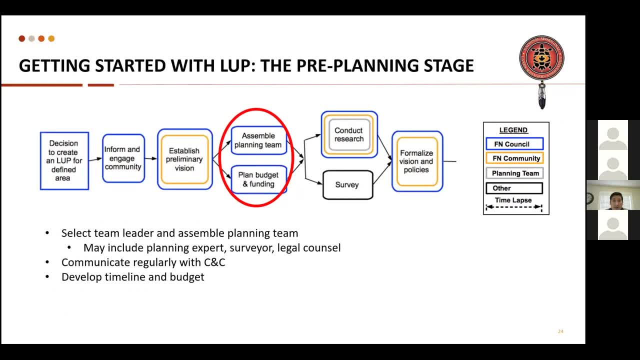 selecting a team leader who's going to spearhead this. so could be your, your Lands Manager, economic development officer and your team. so your team's going to consist of not only local representatives at the First Nation, but time-to-time you might have a planning expert or a 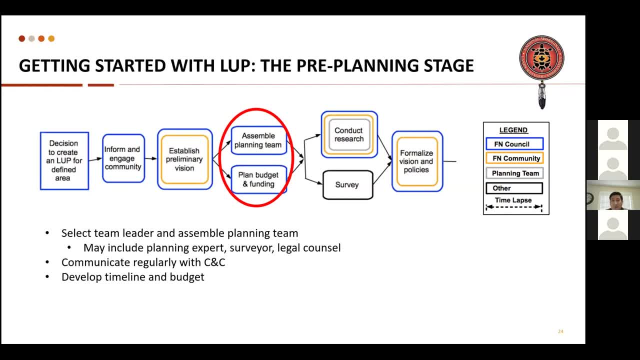 servicing or a legal counsel due to different questions that may arise. so they're not going to come in and sit on every meeting, but if an issue needs to be asked or addressed, you know who. that point of contact is to get answers to some of those questions as part of your committee and then you're going to 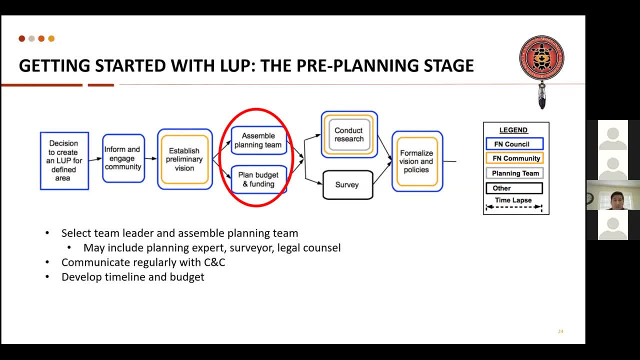 communicate back and forth with your chief and counsel, keep them on the loop, in the loop of the progress that you're making with the land use planning project, and you're going to develop your timelines and budgets. often, if you're looking at a timeline of one to three years, you're going to develop your 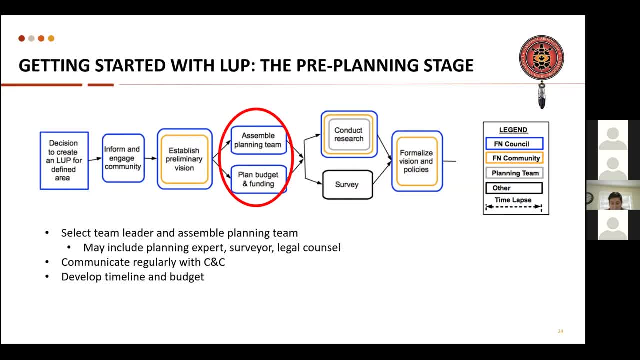 your budget items. often they'll include your First Nation staff, consultant fees, potential, you know, survey cost or legal counsel fees. is the project self-funded by the First Nation or are you going to be looking at other sources of funding? you're going to be looking at other sources of funding. you're going to be. 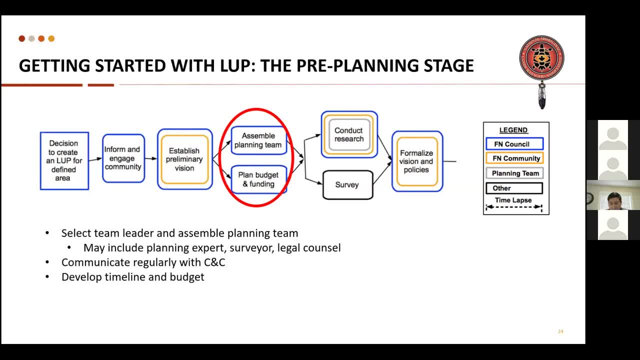 looking at other sources of funding. you know I had indigenous services affairs or your contact Nama for their land use planning funding support or other government or NGO or investment partners. so the next step would be: hey, we want to do this plan, but where are we going to get the money from if it's not? 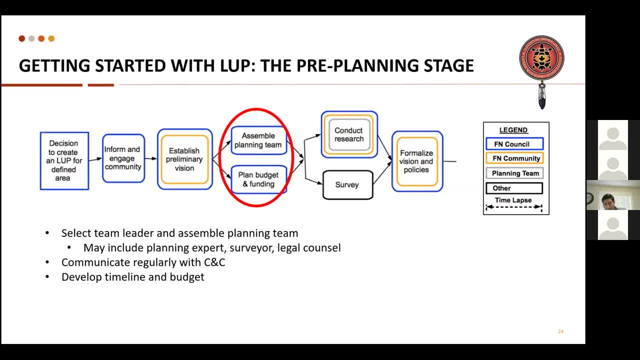 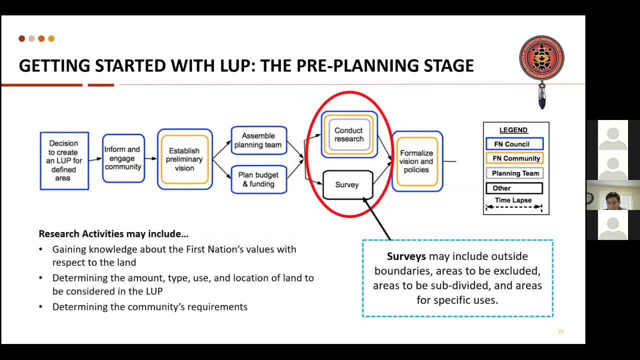 self-funded. on the pre-planning, it's also important to conduct background research, so preliminary background activities can include getting that knowledge about the First Nations values with respect to the land, determining the amount of type and use and location of land to be considered in the land use plan. and 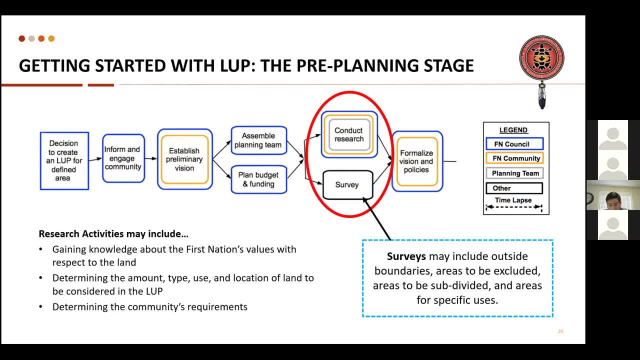 determining the community's requirements. preliminary activities can be studying sections of the the Indian Act in the land use section and requirements of your land regime, for example, our lamp. gaining knowledge about the First Nations values with respect to the land, the lay of the land. also determining land type, land use, location of land that needs to be considered in the land use. 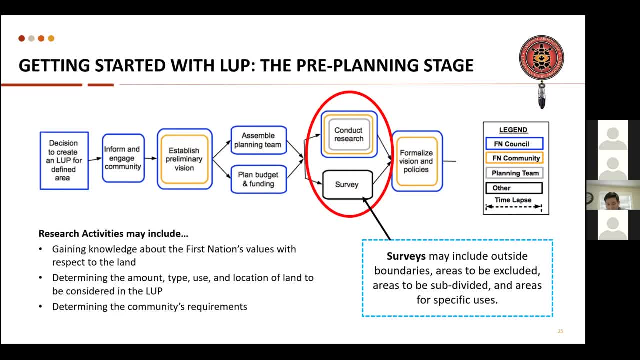 plan, determining, you know what are the community's overall requirements. sometimes you'll be identifying, you know, stakeholders or other interest parties, preparing a suggestion outline for the research report. you can also, for you know, mapping, preparing a sketch of the land for data collection with a view to developing a more detailed 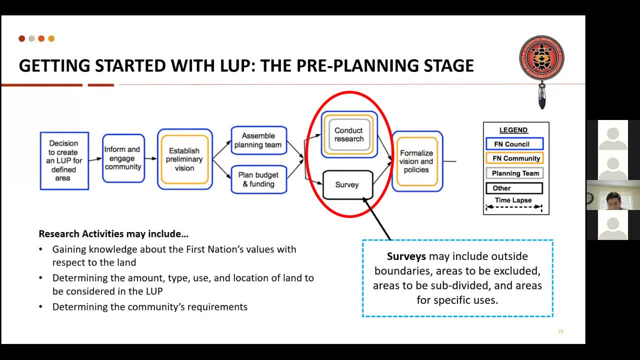 map as you go through the land use planning process. later on you can do survey research questionnaire style. it can be topic specific, such as you know, relating to housing effects, a large burning issue- or it could be economic development in, and have a survey for community members or staff to answer on any other range of topic as well. you can also provide if 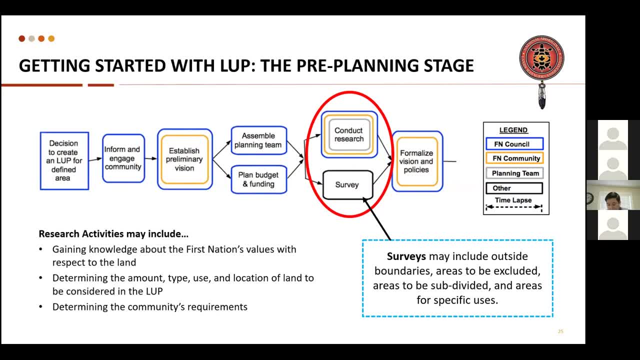 you're looking in, looking at the lay of the land and maps, if you're working with the surveyor, providing maps of different areas, reading these maps or understanding these maps of your subject lanes, looking at, you know where's the residential areas of the community, social, environmental, cái. 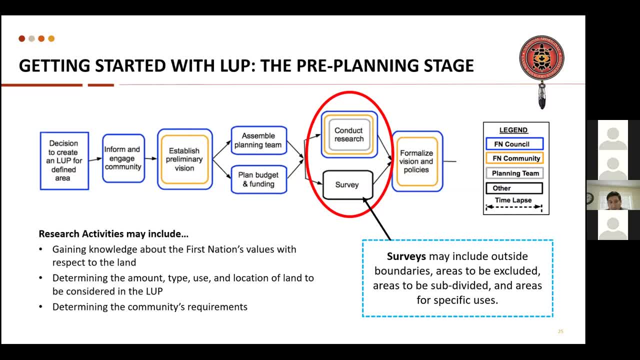 areas, etc. if you're looking at different types of development. what's on the land now? all these are different research activities that you can include at this beginning stage as well. some communities are highly involved with land use, with land surveys, so, um, they'll. they'll do an inventory uh of of their land use currently. you know they're. 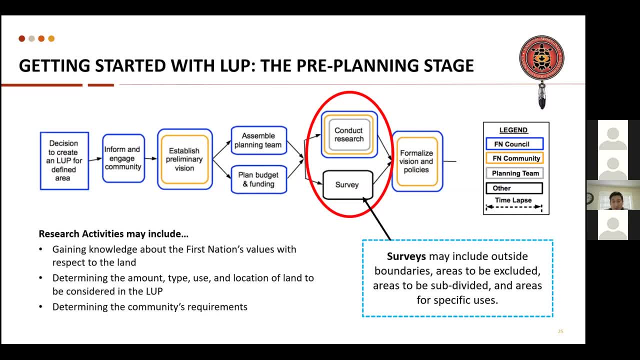 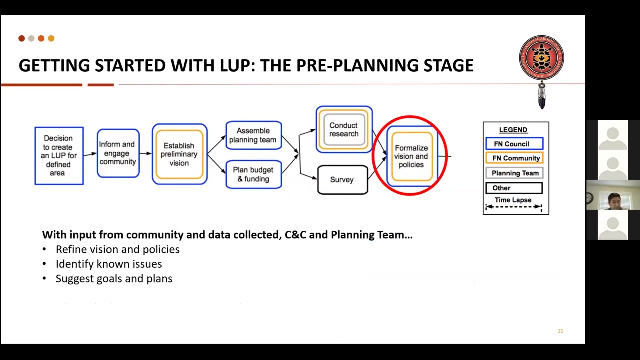 in the reserve boundary line. uh, what survey lands are already divided, subdivided and and used cp lands or banned lands? um, this is just kind of that background researching of of what's on the land currently, uh, of the of your reserve lanes, and that specific use now formalizing visions, policies, with input from your community and data collected. 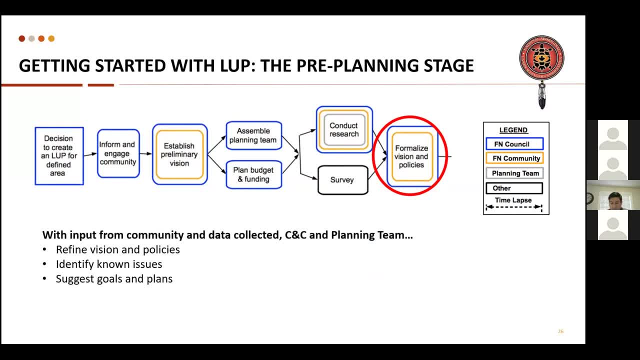 chief and counseling. working with your community planning team. often you'll draft and refine your visions and your policies, identifying any known issues in the community lands, suggesting goals and plans and often, when this stage is complete, you'll have a good background data report of where your first nation community is up to this point, in this point in time, on the lands. 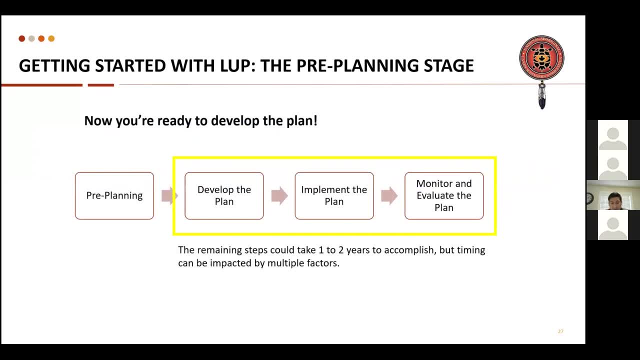 planning process. so that's a lot of the pre-planning. you know kind of where you're at at your local first nation area at that stage, which gives you an idea of how your community may get started with the land use planning process at the beginning steps. however, this is just the 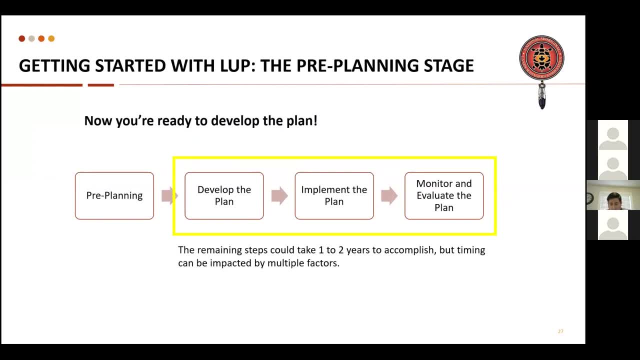 beginning. the next three stages that are in this yellow highlight box here on the screen can take anywhere- about one to two years, uh, to accomplish. on average, the pre-planning stage, as I mentioned earlier, can be three to six months, but developing the actual land-use plan can be about a year on. 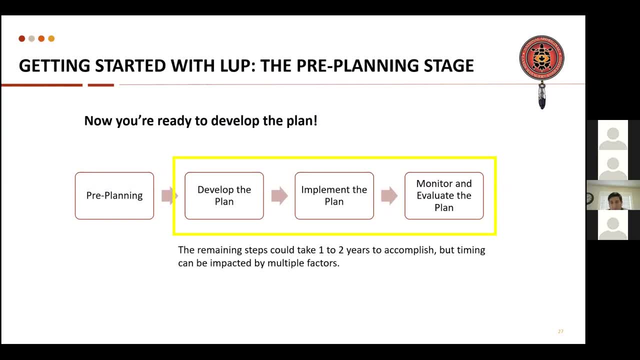 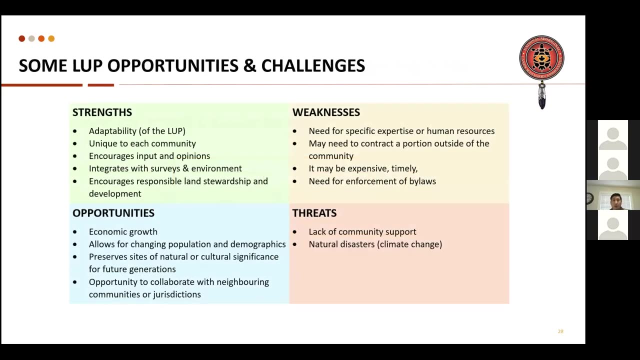 average and then implementing your plan and monitoring and evaluating can take another, you know, three, six or twelve months. it just, it just varies from each First Nation to another Land-use planning opportunities and challenges. so what I have up here is often in summary. I wanted to highlight some possible. 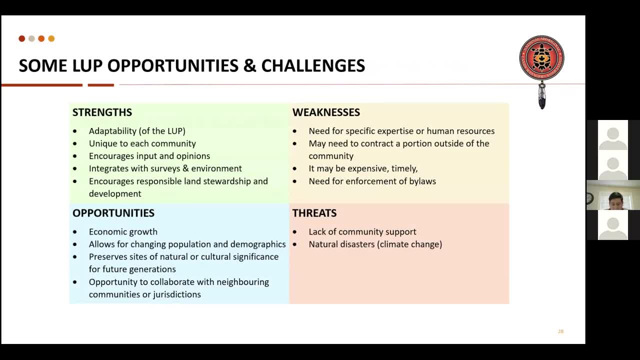 opportunities and challenges that I've heard from First Nation communities over the years. specific opportunities and challenges, of course, differ by each First Nation community as they're faced with their own unique situation. some of the strengths about having a land-use planning opportunity and challenges are. some of the strengths about having a land-use planning opportunity and challenges are. 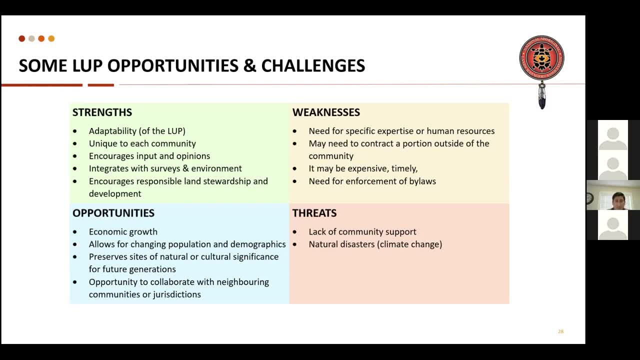 having a land-use plan is having an adaptability of the plan. having where no one land-use plan is the same because it's unique to each of what that First Nation was going through and and where they're heading heading to in the future, encourages input and opinions. integrating that land-use plan with 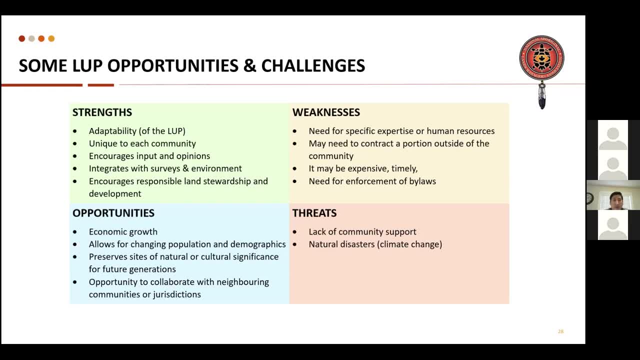 other areas they could, for example, surveys or environment initiatives encouraging responsible land stewardship of your lands and development. some of the opportunities is economic growth and addressing that economic growth through the land use planning process, how your land use plan allows for you know changing population demographics and how you're going to plan and prepare for that at your local. 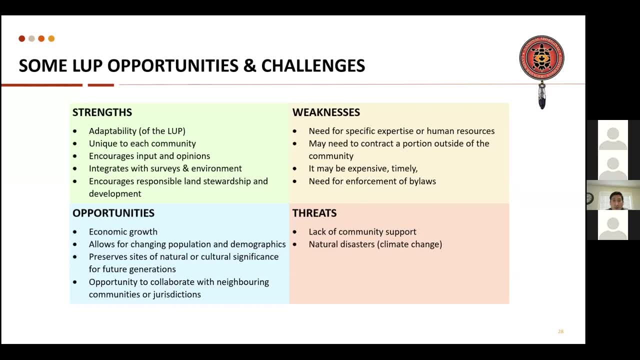 first nation, you might find out that's a younger age cohort and you'll have an emphasis on providing- you know- daycare or schooling services. or you may find out through your statistics, demographics, First Nation level that it's an older aging community and you need to look into additional. 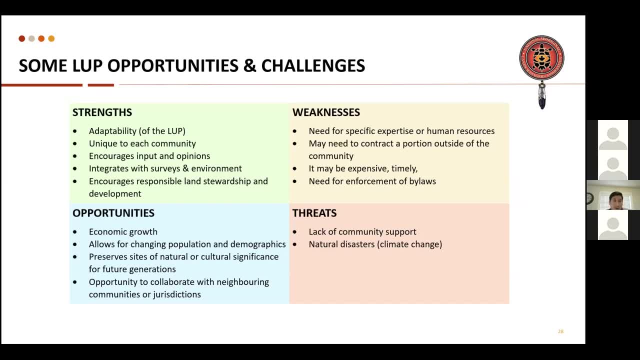 health care services or or providing for your elders. other opportunities is preserving sites of natural or cultural significance for future generations at your local First Nation area. opportunities to collaborate with your neighboring communities or jurisdictions. some communities that are not part of your community are not part of your community, are not part of your community. 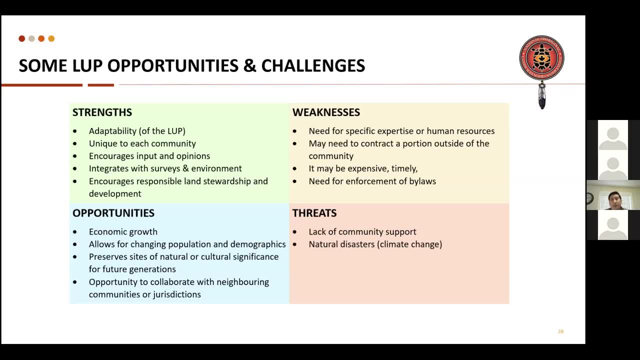 that are nearby a municipal setting sometimes, for example, and they have water issues, that develop inter-municipal agreement or partnership for water sewer. case by case it all depends. but it's looking at those opportunities and not reinventing the wheel. in some cases some weaknesses to land use. 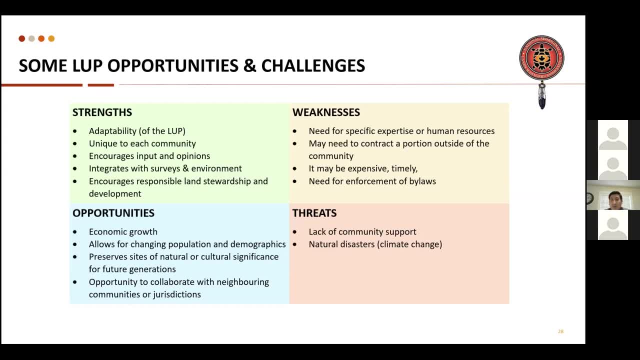 plans that communities have pointed out is a need for specific expertise or, you know, human human resource capital at the nation to assist with it. you may need to contract a portion outside of the community to undertake and complete the land use plan for the community. sometimes you know it can. 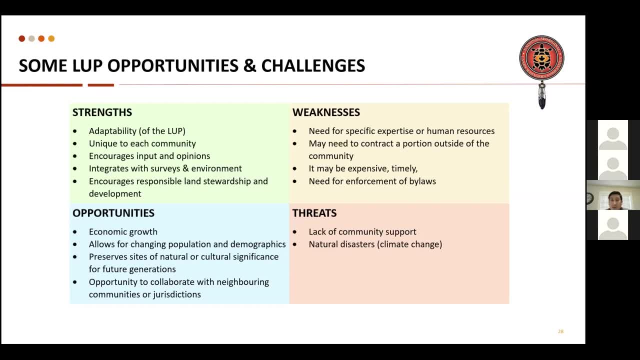 be costly and the First Nation doesn't have the funds to it. so where can they access funding? often also is the need for bylaws, so community may not have any bylaws and as part of the next step for having a land use plan, they would like to do laws or bylaws. 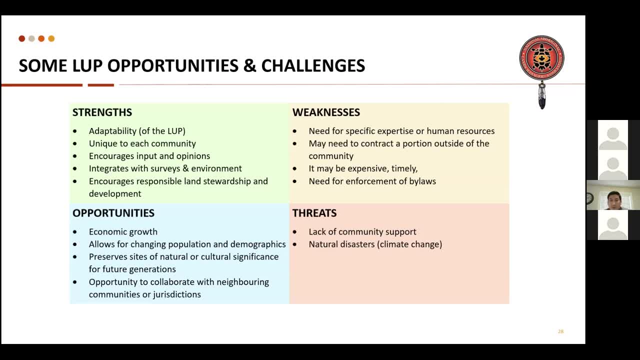 some threats communities talked about is, you know, you might have a lack of community support to do the project. other communities are faced with an increasing, you know, natural disaster and climate change and they see them planning different areas moving forward into the future. but they they're faced with, uh uh, climate change happening and affecting their community in their need to address 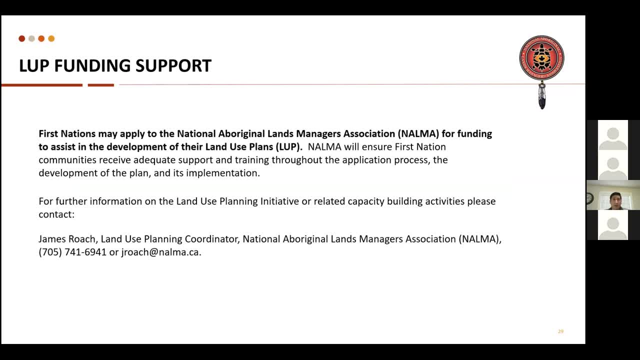 that as well. foreign, foreign, foreign, foreign. so, um, one of the other aspects is: you know where can I get some funding support? one example: First Nations may apply to Nelma. we work with our institutional partners at ISC for funding to assist in communities developing their land use plan. Nelma often, you know, is a 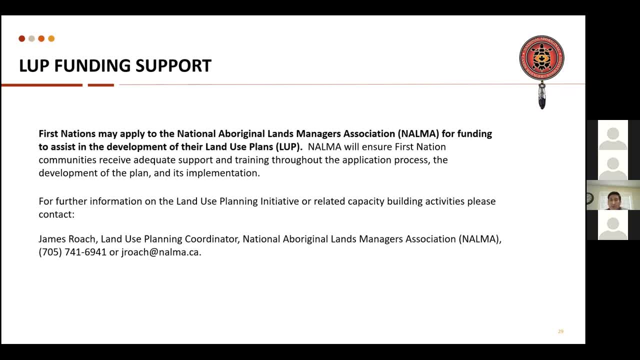 first point of contact to walk the community, the First Nation, through uh in supporting them for adequate funding and support funding. you know time to time is limited but we also provide training throughout the application process. before covid we did our on-site toolkit training but again we're looking at developing new online tools to assist. 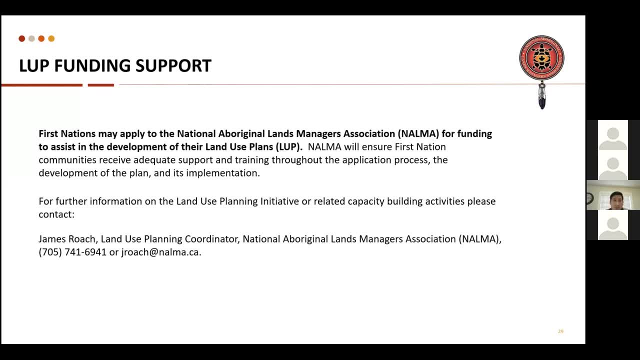 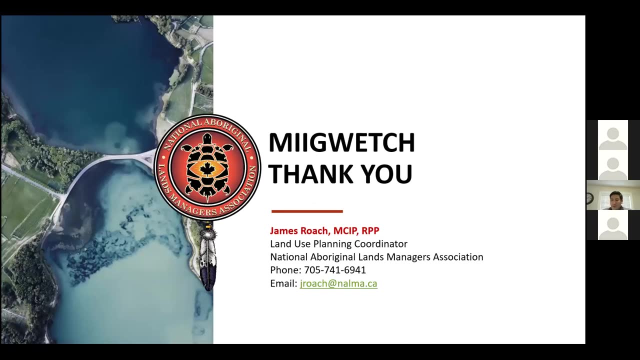 uh throughout the development of the plan in its implementation. you could contact my myself at Nelma. uh, my information is uh, you know, if you go to Nelmaca, my information is there as well. and uh, Miigwech, it's a lot of information uh to get through in this short amount of time, but I 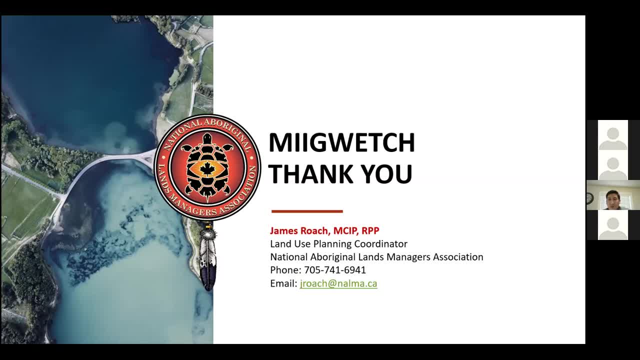 hope we provided you with a little bit of insight for those communities that want a little baseline introduction into uh starting land use plan in their local community areas and gathering some of that background knowledge. thank you, James. I do have one quick question here from one of the participants sure is asking is: 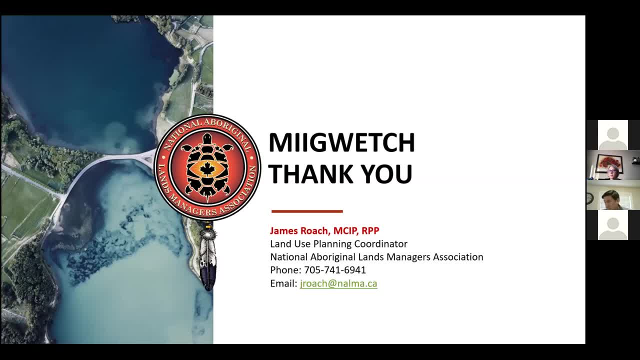 the land use plan a part of a comprehensive Community plant, or is it the same? so, um, often what I'll see is: uh, First Nation communities will do a comprehensive Community plan, uh, uh, and as part of their next step of completing that CCP is they identify to do a land use plan. so their 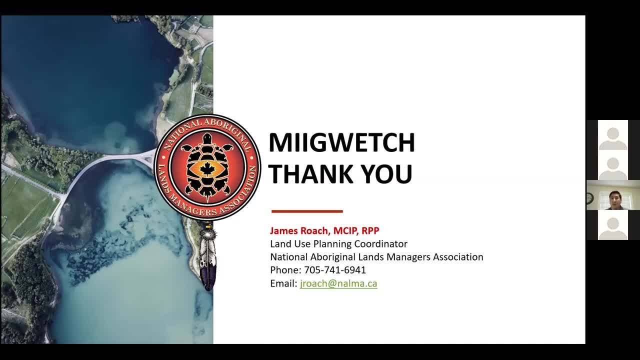 comprehensive Community plan can be all-encompassing, uh holistic view, and then often they'll narrow that down into the land use setting of completing their land use plan. so I'll often see it as a next step, uh uh in the community's process of finishing their CCP and then moving on and and fine-tuning. 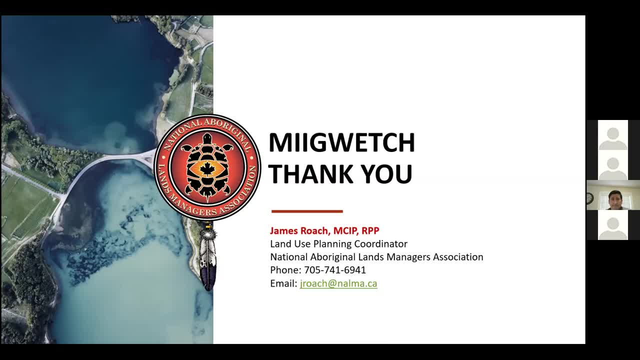 uh in the land use planning form. perfect, thank you. thank you, James, once again for delivering an informative presentation. thank you everybody for attending and I will send a copy of the PowerPoint out to everybody shortly. thank you again and enjoy your day. thank you very much. if you have any questions, please feel free to contact me. thank you, thanks. bye-bye. you. 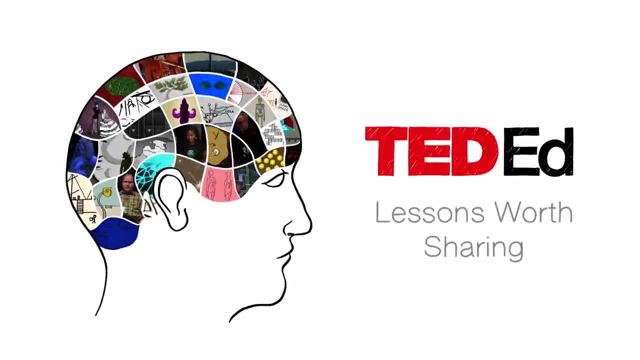 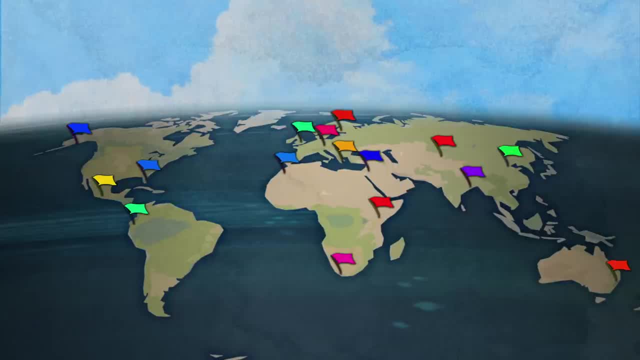 Today, more than half of all people in the world live in an urban area. By mid-century this will increase to 70%. But as recently as 100 years ago, only 2 out of 10 people lived in a city, and before that it was even less. How have we reached such a high degree of? 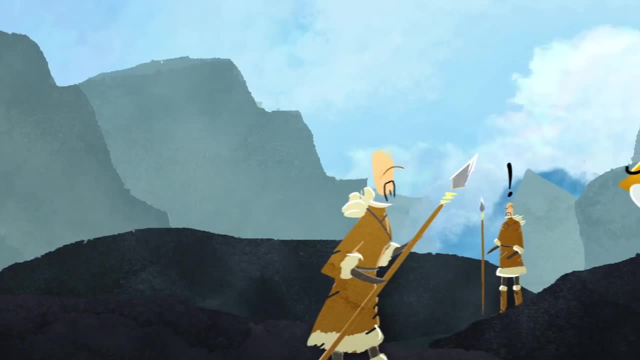 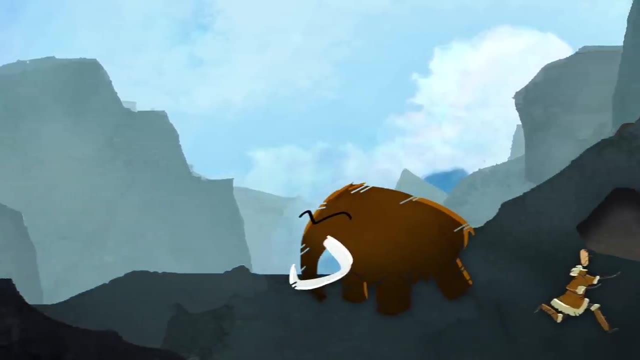 urbanization, and what does it mean for our future? In the earliest days of human history, humans were hunter-gatherers, often moving from place to place in search of food. But about 10,000 years ago, our ancestors began to learn the secrets of selective breeding. 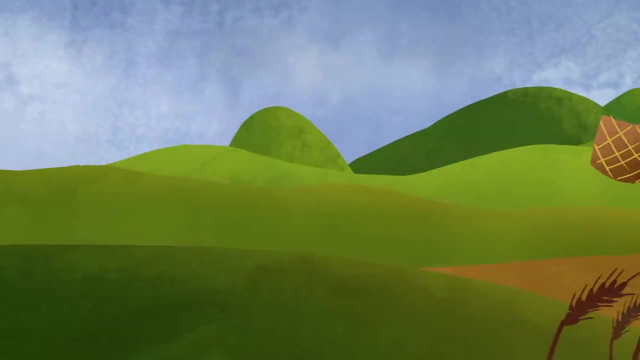 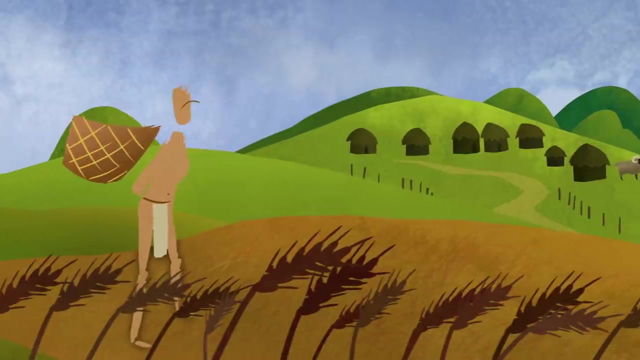 and early agricultural techniques. For the first time, people could raise food rather than search for it, and this led to the development of semi-permanent villages for the first time in history. Why only semi-permanent, you might ask. Well, at first the villages still had. to relocate every few years as the soil became depleted. It was only with the advent of techniques like irrigation and soil tilling, about 5,000 years ago, that people could rely on a steady and long-term supply of food, making permanent settlements possible. And with the food surpluses that these techniques produced, it was no. 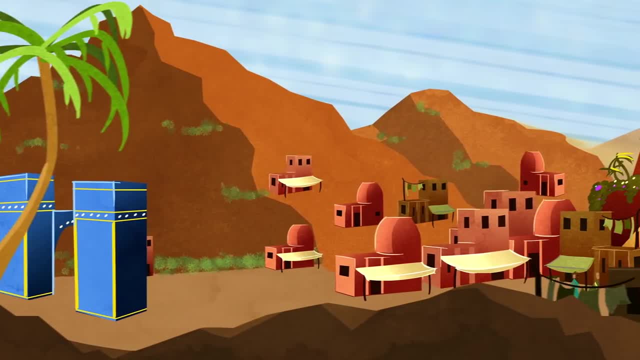 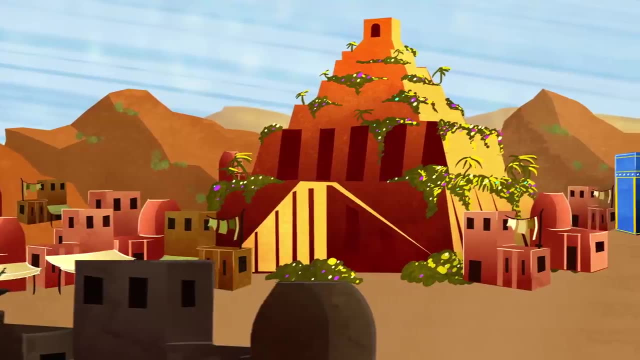